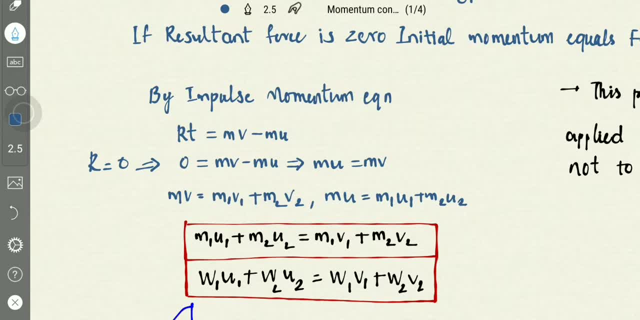 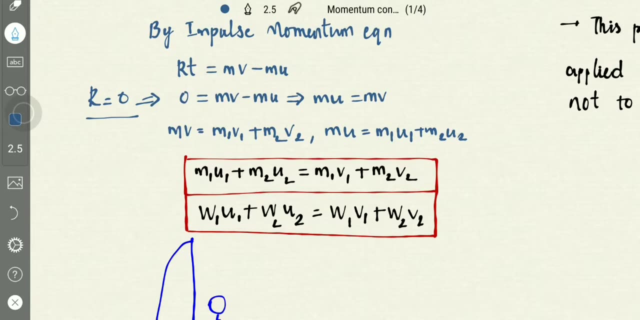 this is what the statement is saying. If resultant force is equal to zero, the initial momentum is equal to final momentum. If there are two bodies, then it will be. the final momentum will be m1 v1 plus m2 v2.. This is the final momentum of first body and this 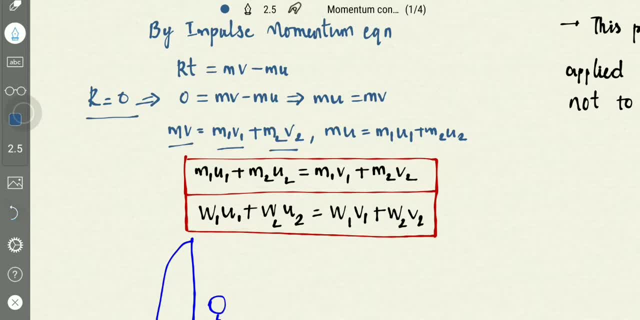 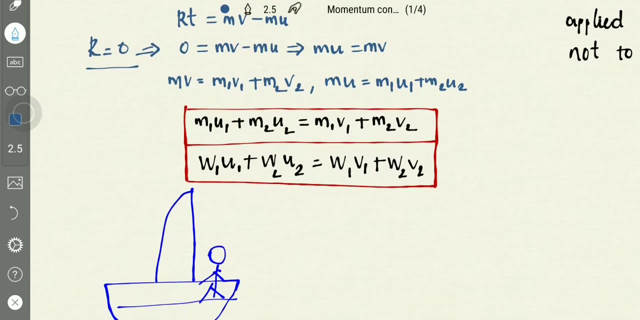 is the final momentum of second body And this will be total initial momentum will be initial momentum of first body and initial momentum of second body. If you write here m1 u1 plus m2 u2 is equal to m1 v1 plus. 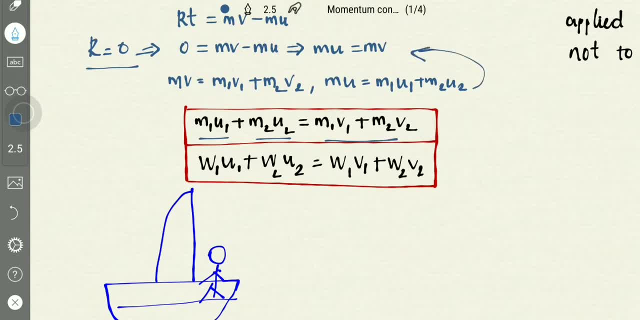 m2- v2. if you substitute this in this equation- And we can also write this as m1- can be written as w1- v2.. divided by g, right, which is equal to m1, so we can represent this equation in terms of w also, because all the g's in the denominator will gets cancelled, so we can represent in: 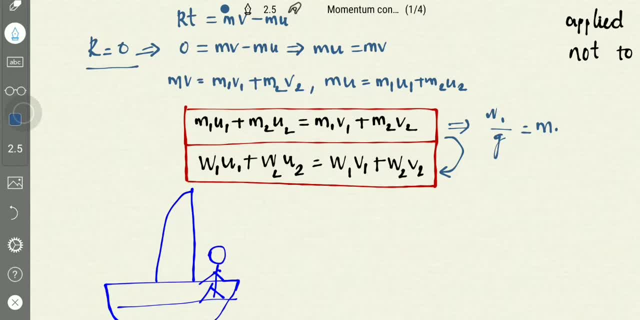 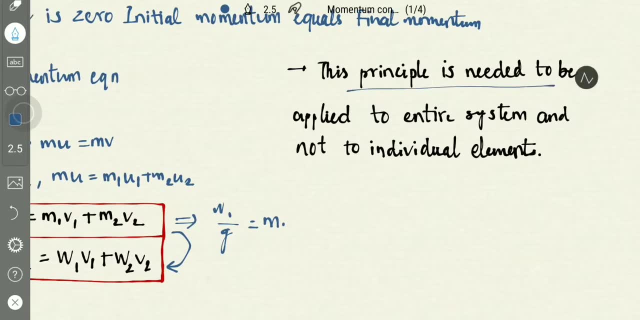 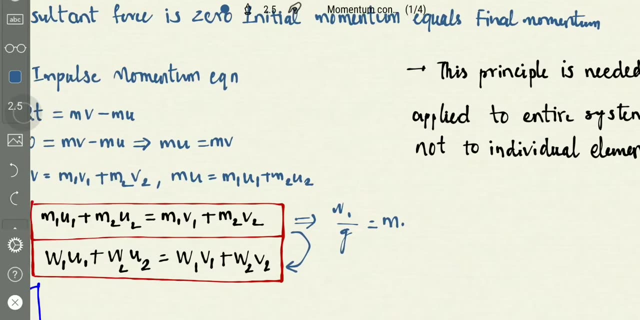 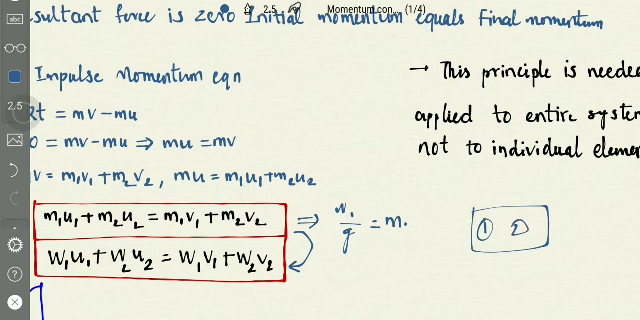 terms of weight and also in terms of mass. so again, an important point it is saying is: this principle is needed to be applied to the entire system and not to the individual elements. see, we have seen there are two bodies here, and if a system has two bodies and this, 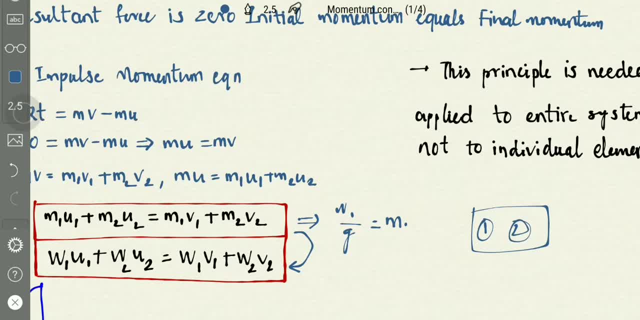 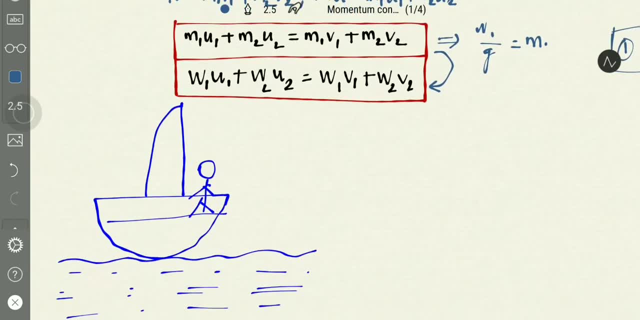 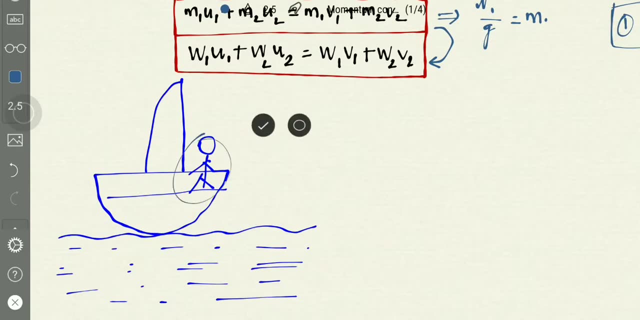 conservation principle should be applied to the whole system and not to the individual bodies. So let us take this example and we apply this conservation of momentum. So a guy is there who is standing in the ship and he is trying to jump into the water in. 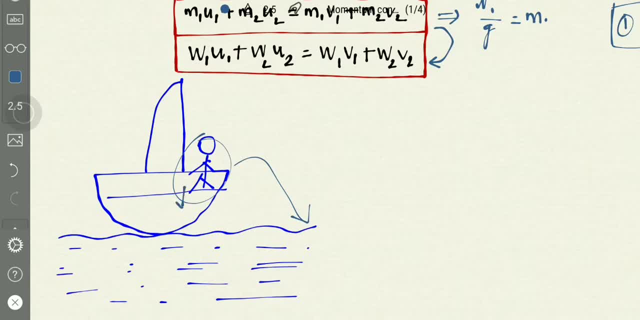 order to jump, he first applies force here. due to this application of force, the water exerts a reaction on the ship. so this force and this force gets balanced. so f-r, considering the upward forces as positive f-r, is equal to zero. so the resultant is resultant is equal to zero. so then we can. 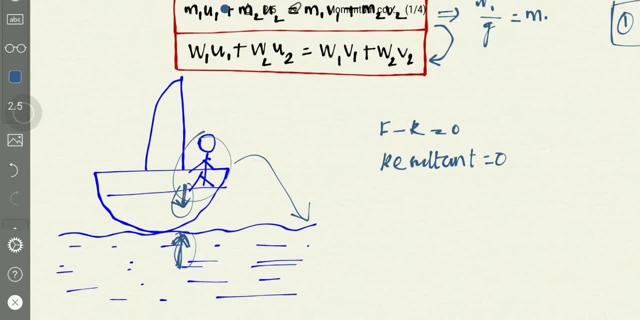 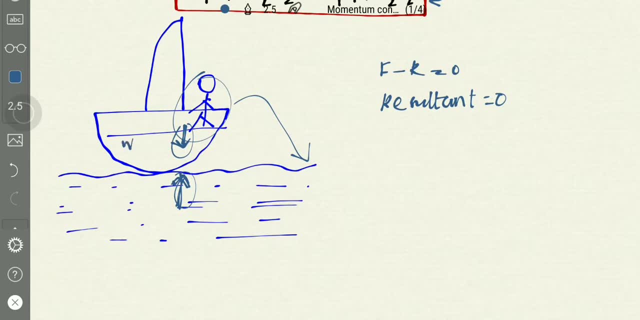 apply here conservation of momentum principle. suppose that the ship has mass m1 and this guy has mass m2. So before jumping, let us say the ship is moving with the velocity of u and say after travelling a distance, after jumping, he jumped into the river. let us say now the ship has 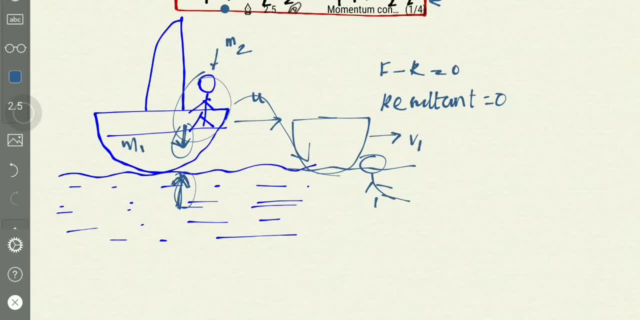 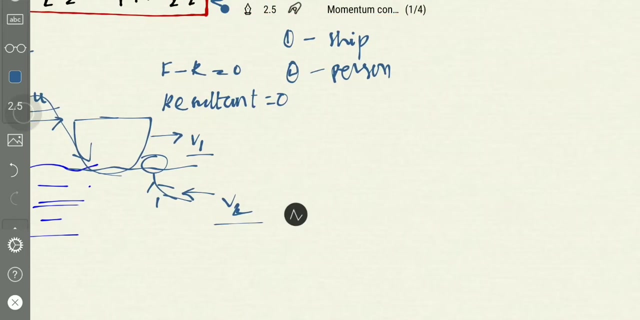 velocity v1, which is final velocity, And this guy has velocity v2.. So here, first body is ship and second body is person. Firstly, initial velocity of ship and the person is same, which is u, and when coming to the final, the ship has velocity v1 and the guy has velocity v2. as the resultant is zero, we can apply conservation. 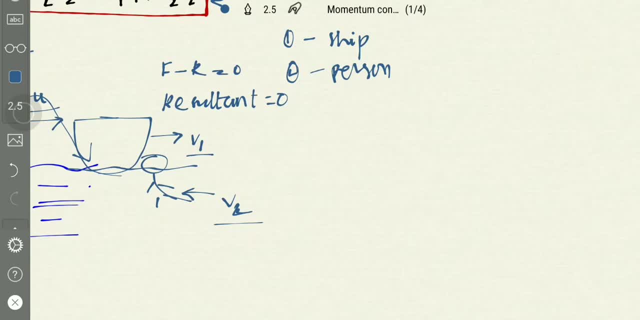 of momentum. So what is conservation of momentum? principle m1, u1 plus m2, u2, total initial momentum is equal to total final momentum, m1, v1 plus m2, v2. so here m1 and m2 are different, but u1 and u2 are same because they are the man and the ship is has the same velocity. so m1 plus. 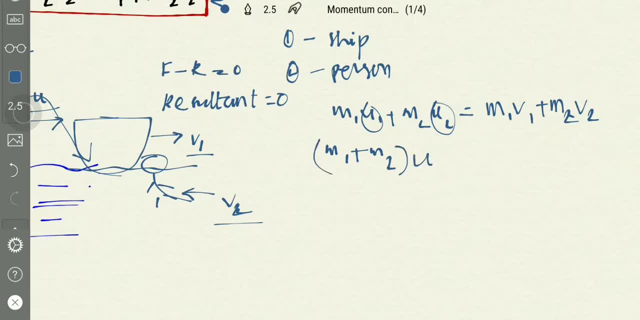 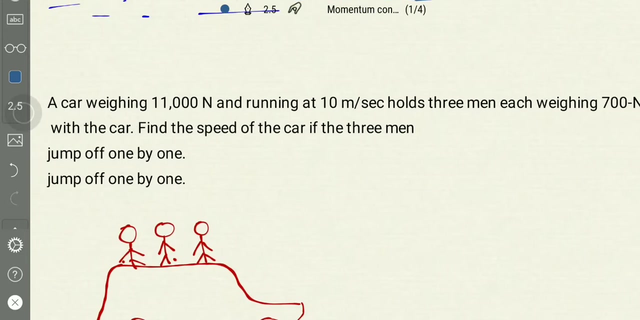 m2 into taking the u as common, because u1 is equal to u2 is equal to u, and here m1 v1 plus m2 v2. so this is how we need to apply the conservation of momentum principle. Let us solve the problem based on this conservation of momentum. 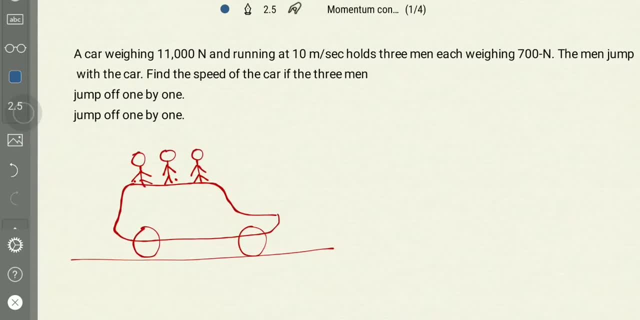 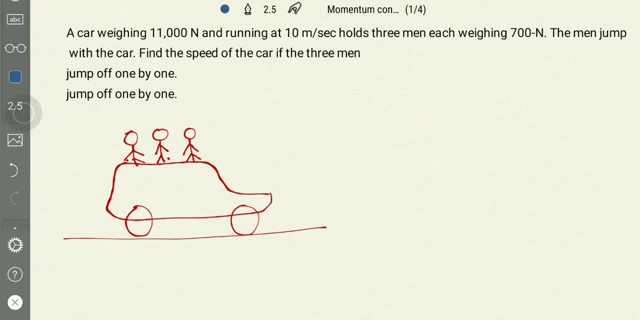 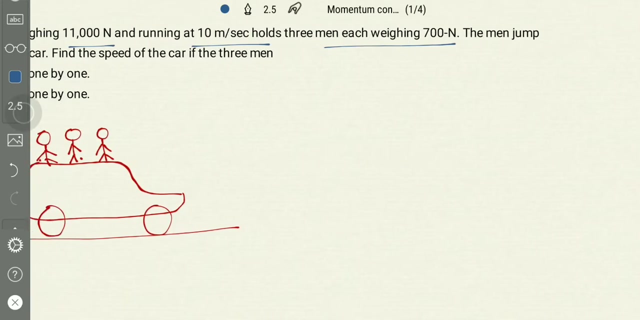 Thanks for watching. So here a question is given. a car is weighing 11000 newtons, running at 10 meter per second, holds 3 men weighing 700 newtons. the men jump. the question is: there are 3 men on? 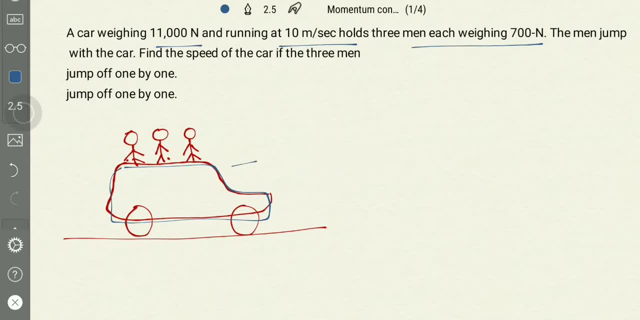 this car and this car is travelling at 10 meter per second. when 3 are on this car, Ok, And each person jumps one by one, and the relative velocity between car and this person is 5 meter per second. What is relative velocity? 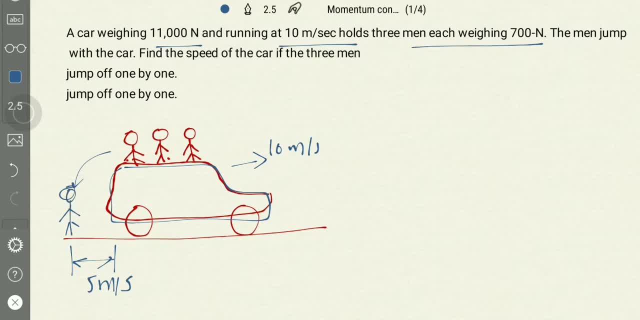 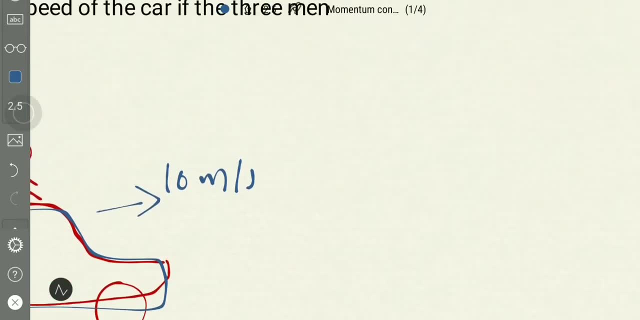 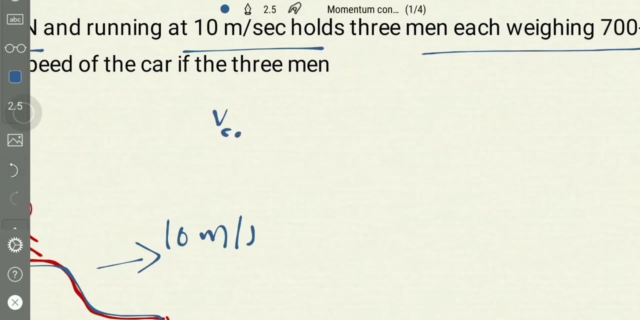 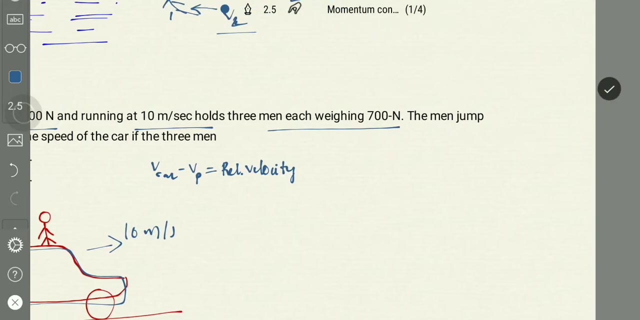 Velocity of this person when compared to this velocity, which is called relative velocity. So we can write so: velocity of car, Velocity of car minus velocity of person, is equal to relative velocity in this case. Relative velocity in this case is this: 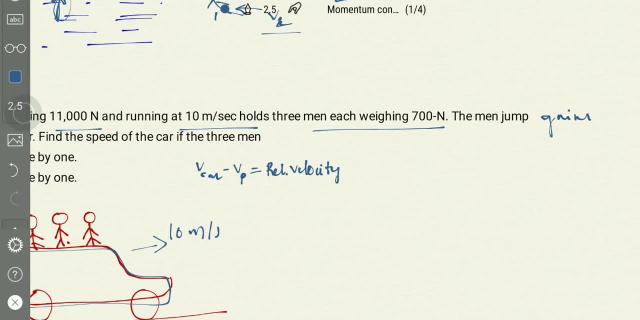 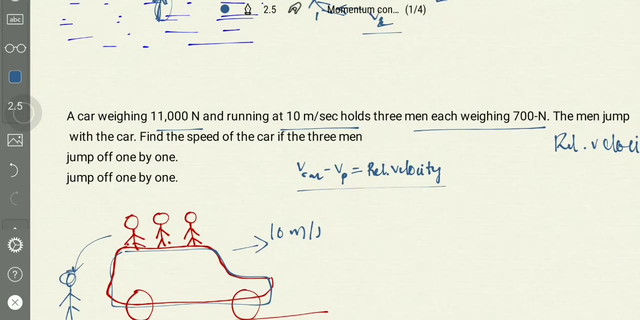 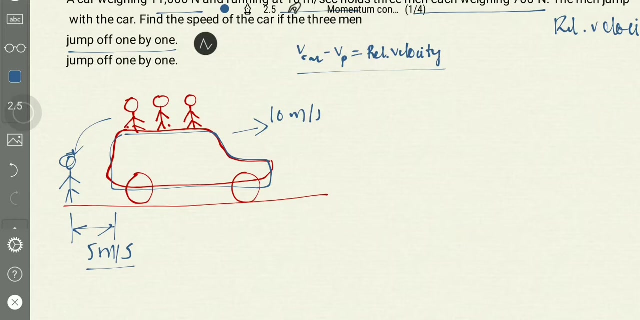 The men jump, gaining relative velocity 5 meter per second. 5 meter per second, then this is the relative velocity. Find the speed of the car if 3 men jump jump off one by one. If one man jumped off, the velocity of this car increases to a slight extent, and if another, 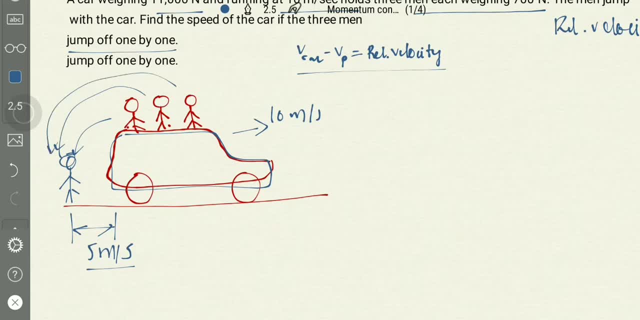 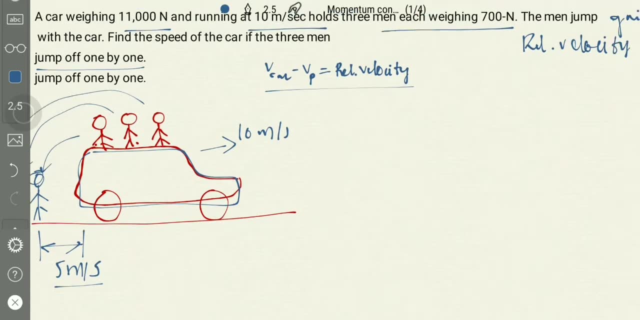 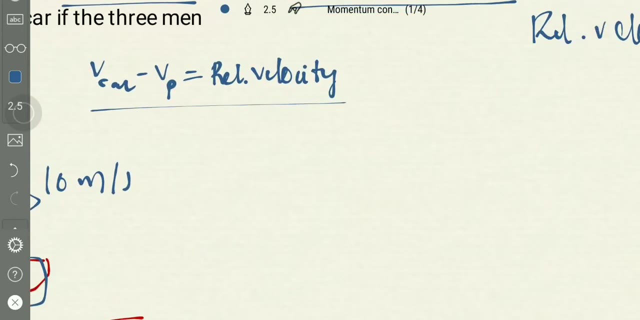 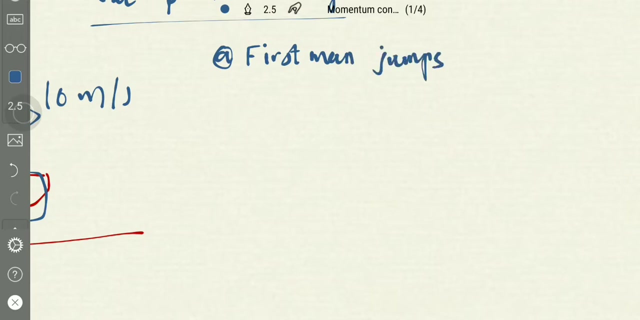 man jumps and the velocity increases. and if another man jumps and again the velocity increases. So what is the final velocity by each jump? So in order to find this, we need to apply this conservation momentum principle. So, firstly, let us say: first man jumps. 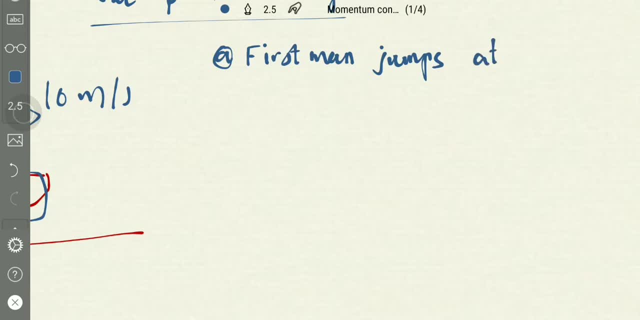 First man jumps off at V1 meter per second. So if the first man jumps off, the car will be moving with a speed of V1 meter per second. After jumping, the car will be moving at V1 meter per second. The initial velocity is U is equal to 10 meter per second. 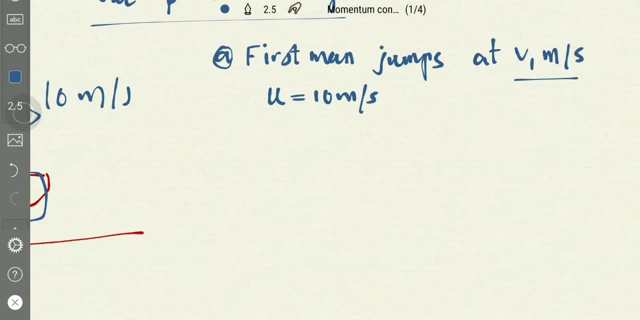 And now let us apply the conservation of momentum. What is conservation of momentum? Initial momentum, What is initial momentum? W1 U1 plus W2- U2 is equal to W1- V1 plus W2- V2.. And here the W1 is 11000. 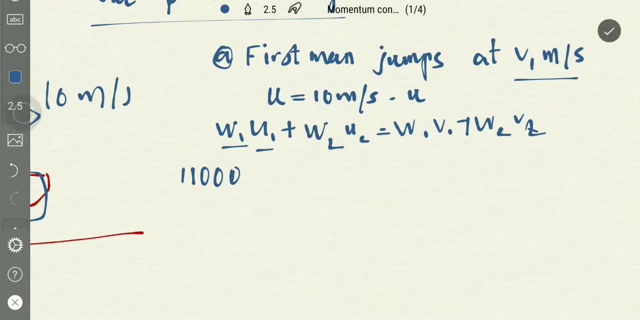 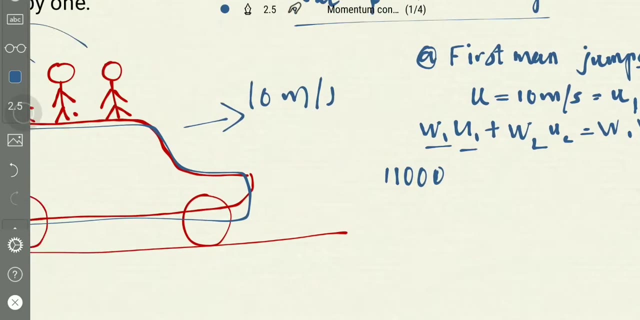 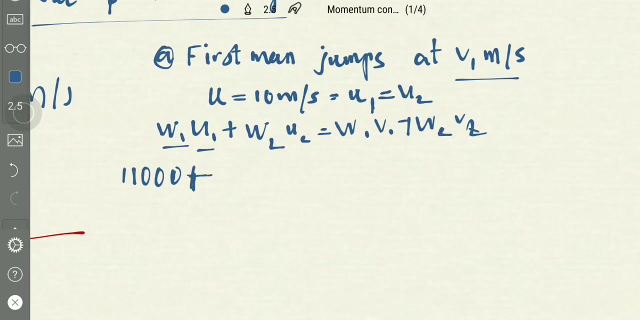 And here U1 is equal to U2, which is U1 is equal to U2.. Because the three people and the car is travelling with same velocity, because they are sitting on the car. So, taking U common and W2, weight of each person is 700 Newton. 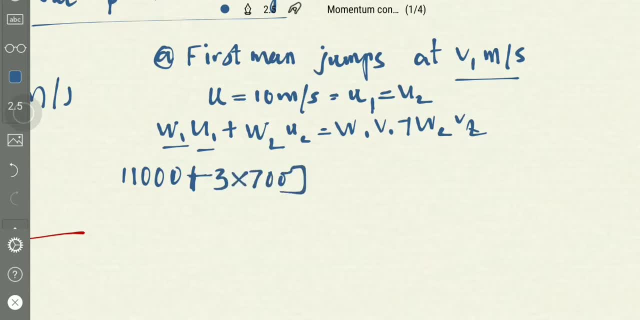 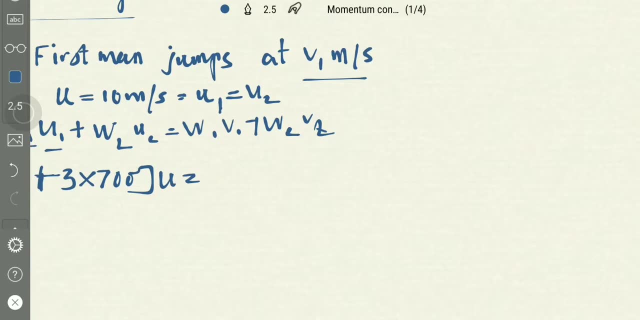 So 3 into 700 into U is common, which is equal to Here. weight of the car is 11000 Newton. And finally, there are two persons sitting here But one person is running on the road. So the total weight of the car after he is jumping on the road is 2 into 700. 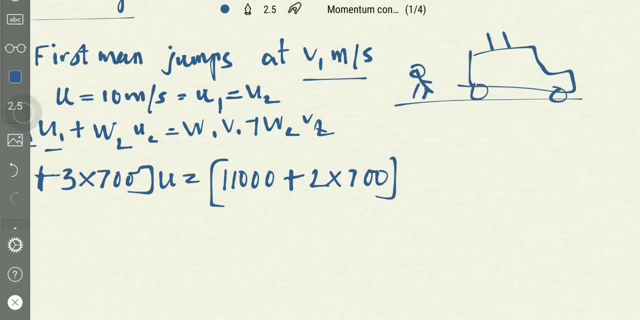 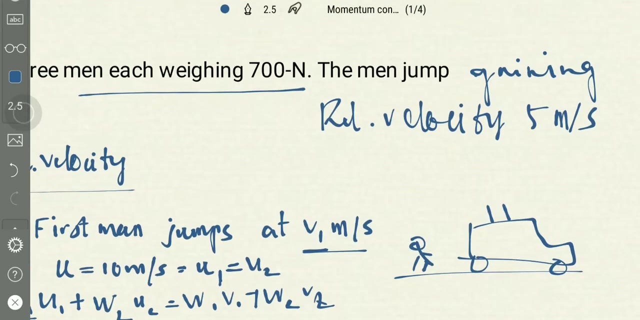 Because only two members are on the car, The velocity with which the car is travelling after the first man jumps is V1.. This is V1. And velocity of the person running on the road is V1 minus 5. Because relative velocity is car velocity minus person velocity. 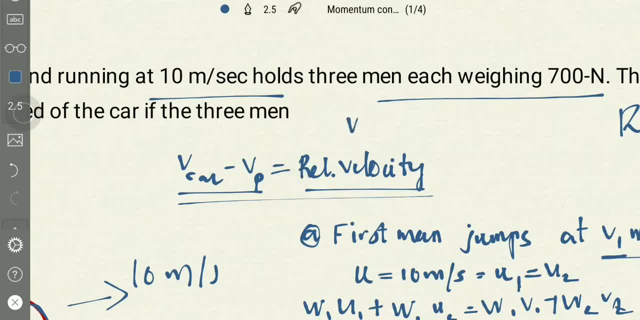 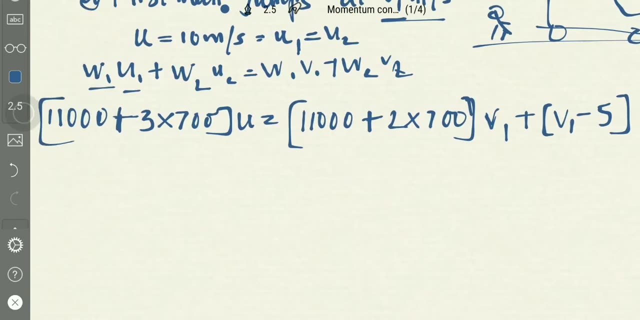 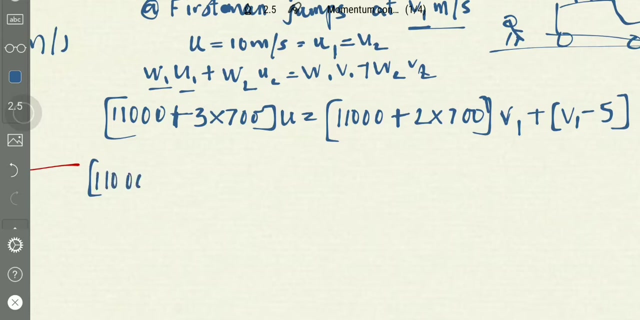 So we need person velocity right. Vp is equal to Vcar minus relative velocity. So car velocity V1 minus relative velocity is 5.. So here U is 11000 plus 3 into 700 into 10 is equal to. 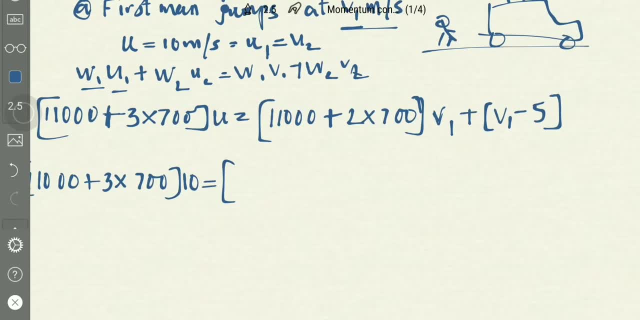 Here there is 2 into 700 into V1. And here it is 1 V1.. And if we take V1, common from these both 11000 plus here 2 into 700, into V1. And again here it will be 700 here. 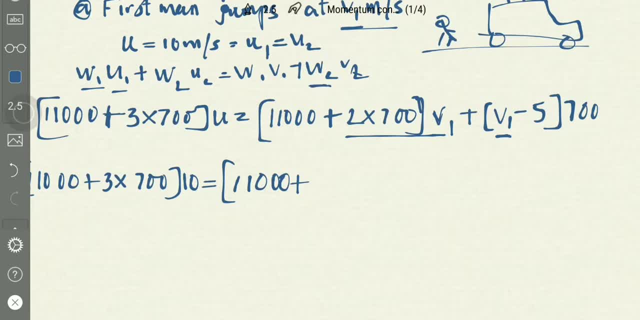 Because W2 is 700, the weight of one person, W2 is 700.. 11000 and 700 into V1 plus 2 into 700 into V1. Which will be 3 into 700 into V1 minus 5 into 700.. 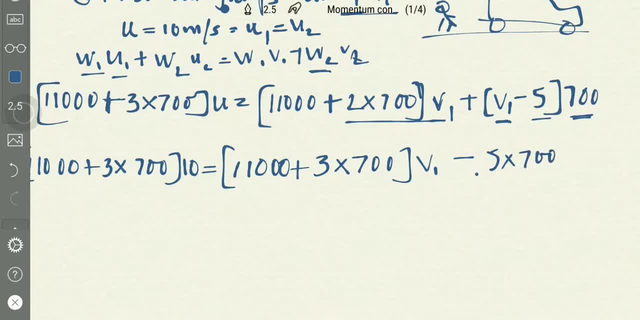 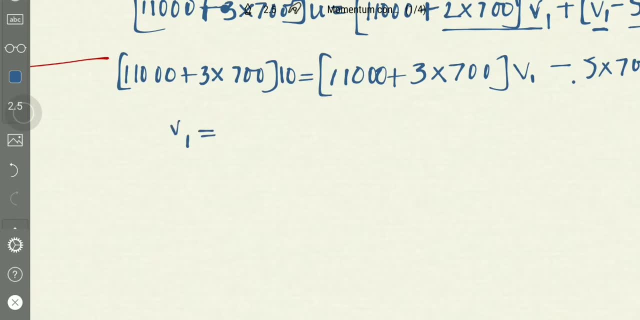 5 into 700.. From this we can find V1, as V1 is equal to 700.. If we simplify this, it will become 700 into 5, divided by 11000 plus 3 into 700 plus 10.. This will be the V1.. 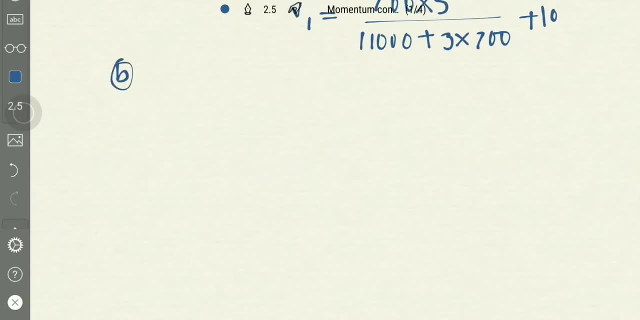 So next one, Second person. Second person jumps off, Second person jumps at, let us say, V2 meter per second, Which means after second person jumping the car travels with the velocity. Here it is traveling with velocity V2.. 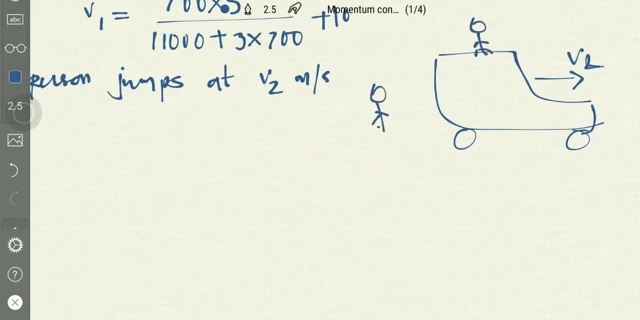 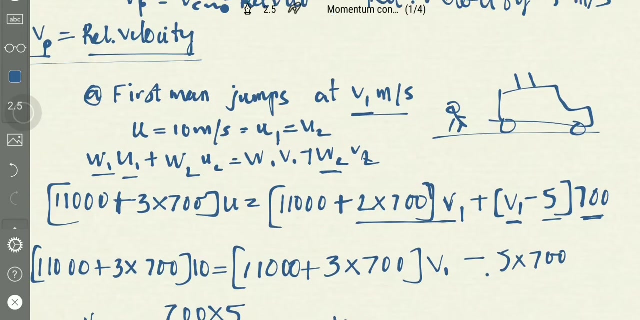 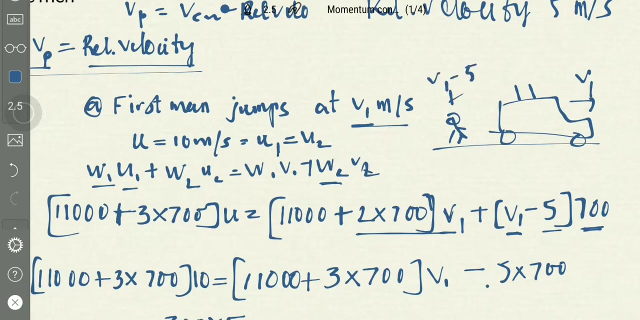 Only one person is sitting on the car. The second person is running here, And the second person is running with the velocity V2 minus 5.. 5 is relative velocity. Here the car is traveling with the velocity V1.. And this person is traveling with the velocity V1 minus 5.. 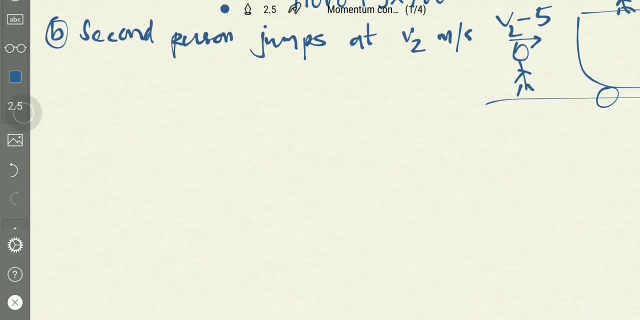 So the initial momentum is: Firstly, 2 persons are on the car. 2 persons are on the car initially, So 11000 is the weight of car, plus 2 persons are on the car, Each of 700 Newton weight. 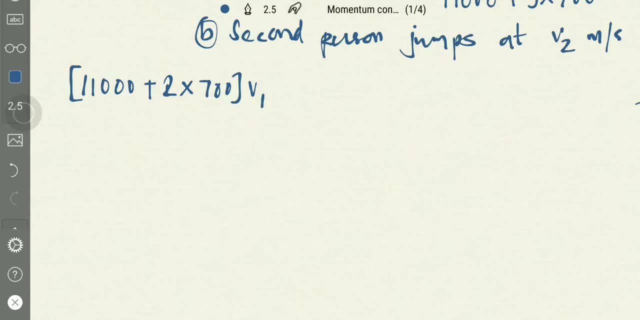 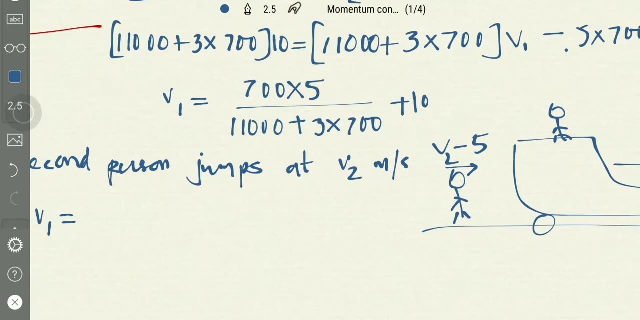 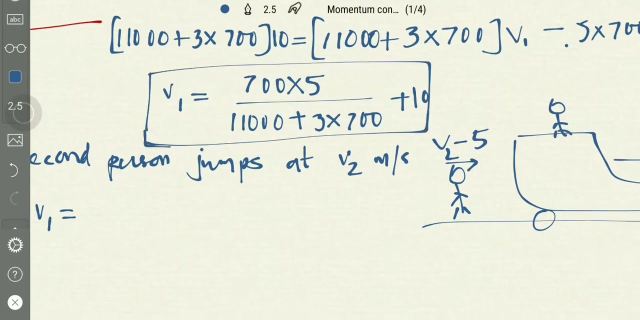 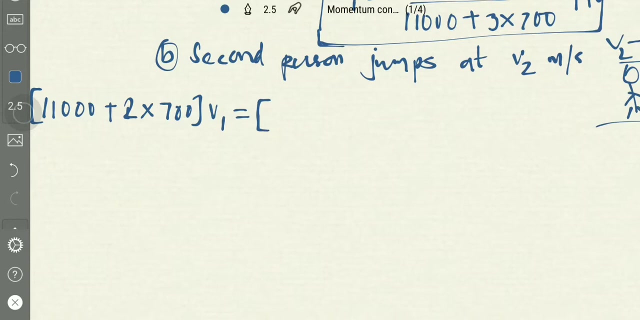 The initial velocity will be V1.. Why it is V1? Because After jumping, After jumping of the first person, The final velocity is V1. So for the second person jumping, The initial velocity will be V1.. And 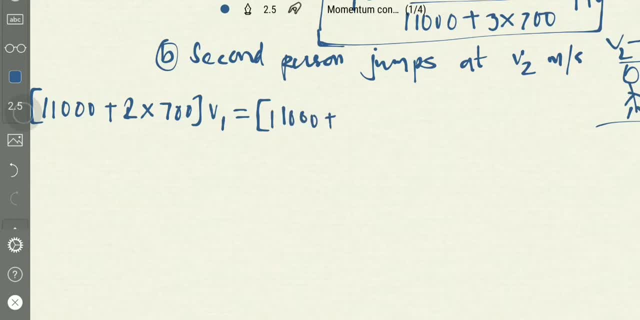 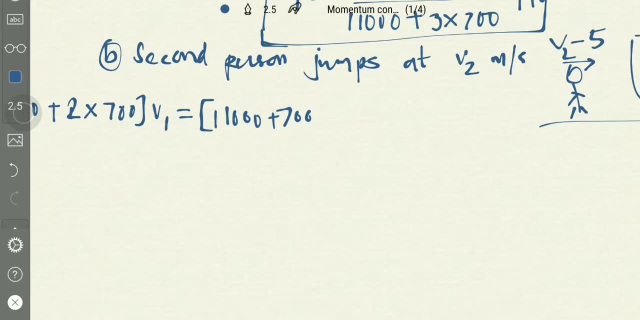 Weight of the car is 11000.. And after jumping of the second person, Only one person is left on the car. So the weight of that person is 700.. And the car is traveling with the velocity V2. Plus And the weight of the person. 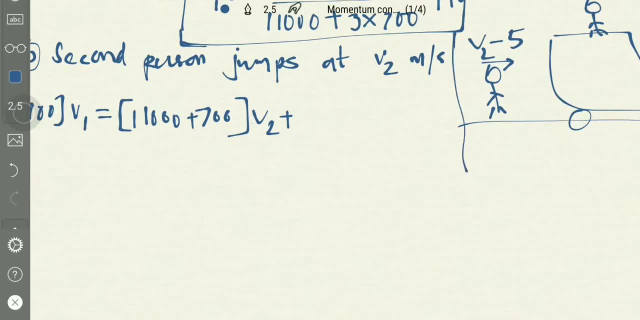 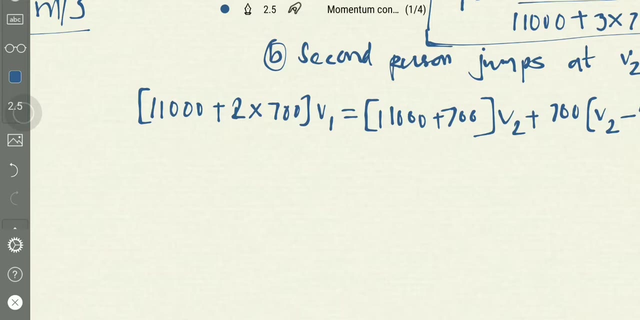 The second motor, right Weight of the person is 700.. Velocity with which he is traveling is V2 minus 5.. Ok, From this, If you solve this, 11000 plus 2 into 700.. Into V1 is equal to 11000 plus. 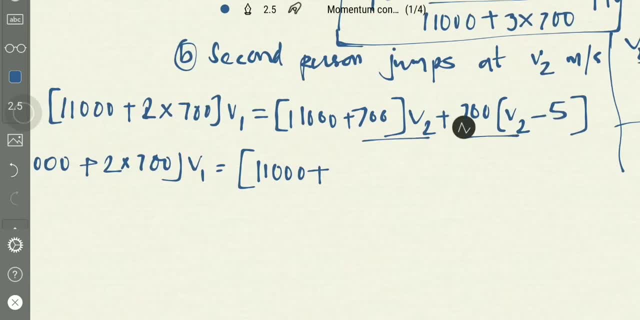 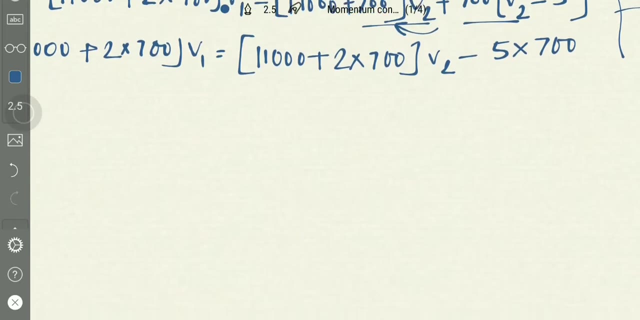 Here it is 700 V2, and here it is 700 V2.. If you take this V2 into this one, So it will become 2 into 700.. Into V2.. Minus 5 into 700.. So it becomes now. 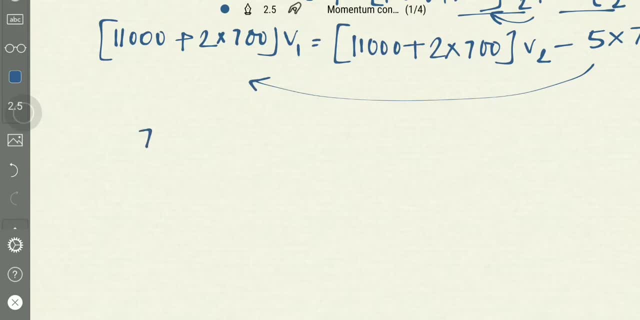 Here: Sending this to this side, 700 into 5 is equal to, And sending this to this side, 11000 plus 2 into 700. Taking common And here it will be V2 minus V1.. So sending this to this side, 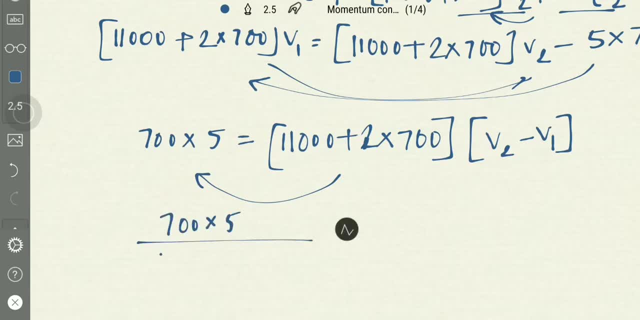 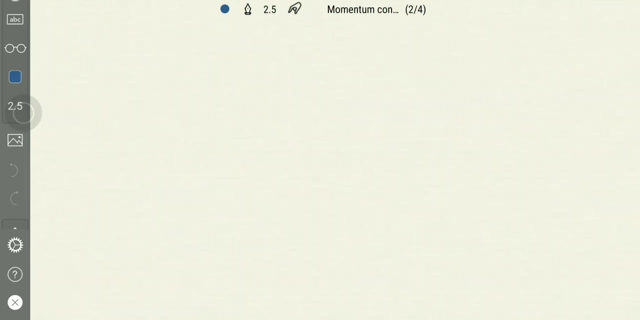 700 into 5.. Divided by 11000.. Plus 2 into 700.. Plus V1.. Gives V2.. Ok, This is V2.. And next We got V2.. And the third person should jump. So third man. 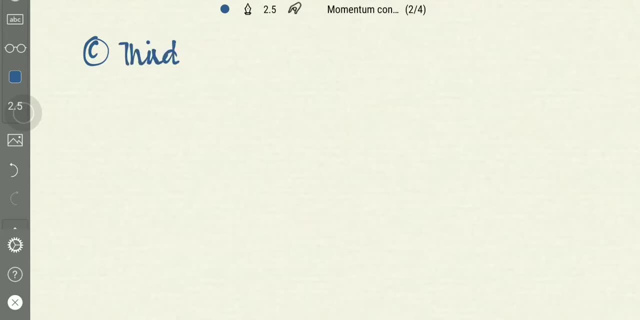 Third person Jumps off it. Let us say, V3 meter per second. This is what we need to get right. This is the car And no one is present on the car now And the person is jumped here. The velocity with which he is travelling is. 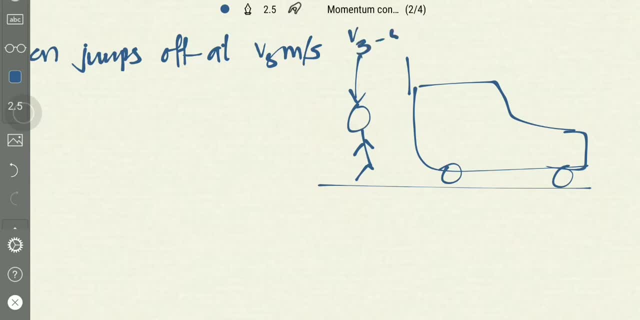 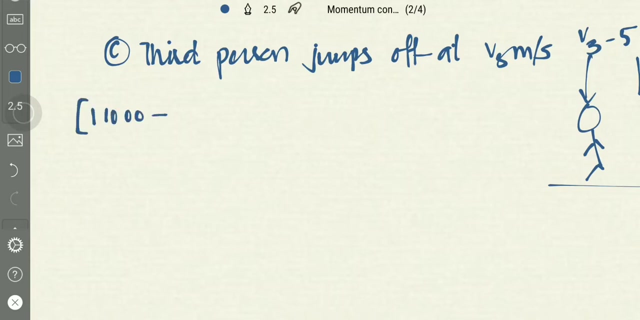 V3.. V3 minus 5 meter per second. This will be travelling with the velocity V3. So initially The weight of the car is 11000.. Plus, With one person, 700. And it is travelling with the velocity. 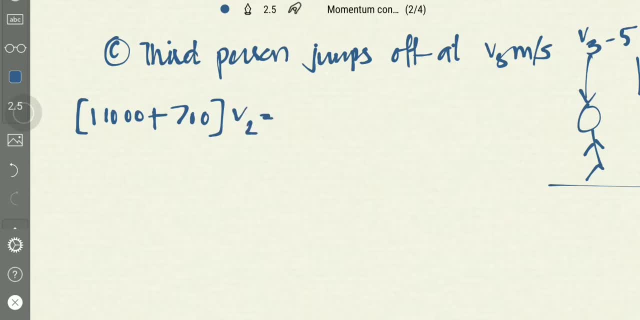 V2.. Finally, Car weight is 11000 Newton Into velocity with which it is travelling is V3. And the velocity of the Sorry Weight of the person is 700.. Velocity of the person with which he is travelling is: 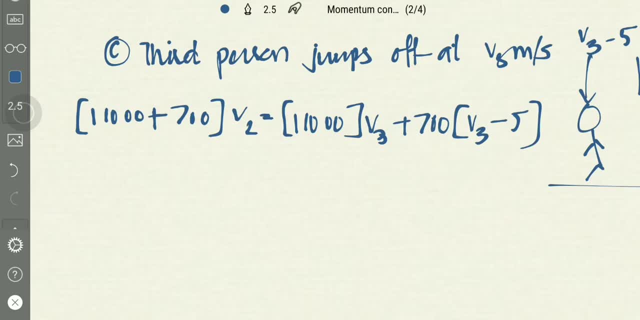 V3 minus 5.. If we solve this, 11000. Plus 700. Into V2. Which is equal to 11000 V3 and 700 V3. So we can Get here as 11000 plus 700.. 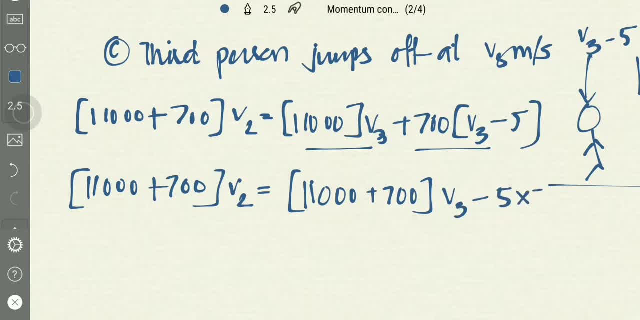 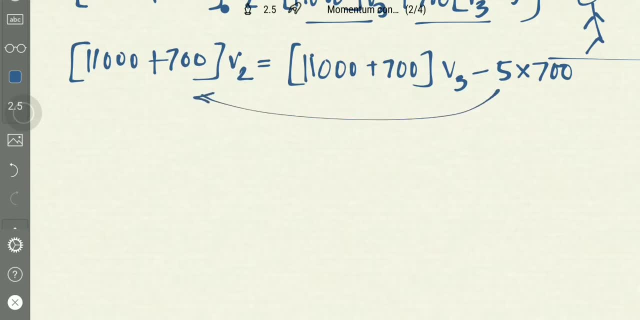 Into V3. Minus 5 into 700.. And from this, If we send it to here And this to here, 5 into 700 is equal to This. two are This, two are same And we can take common. 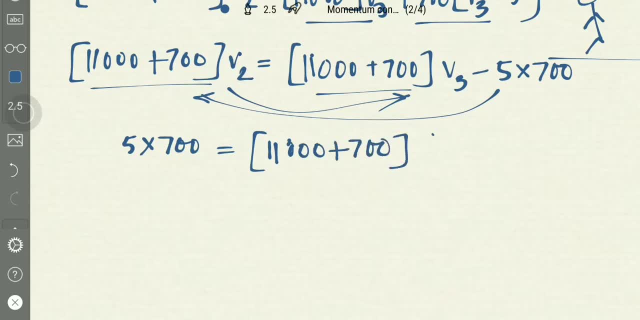 11000 plus 700.. Into V3 minus V2.. Again, sending this to this side: 5 into 700 divided by 11000. Plus 700.. And sending this also to this side, Plus V2.. Gives V3.. 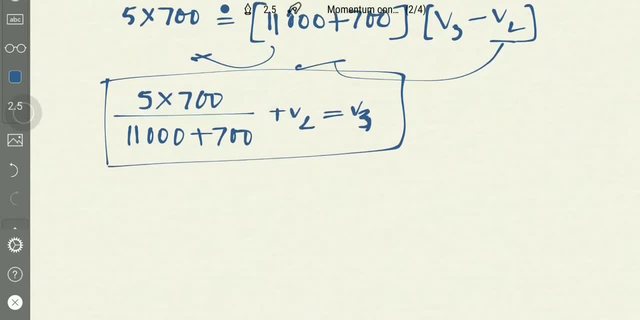 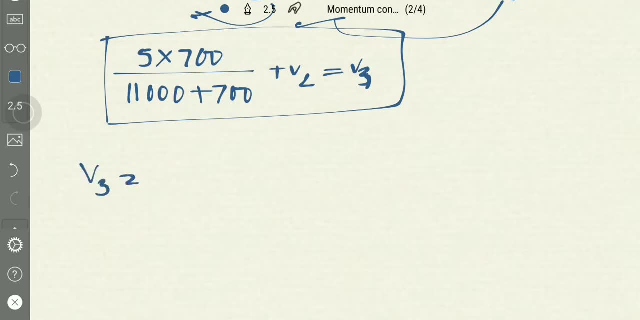 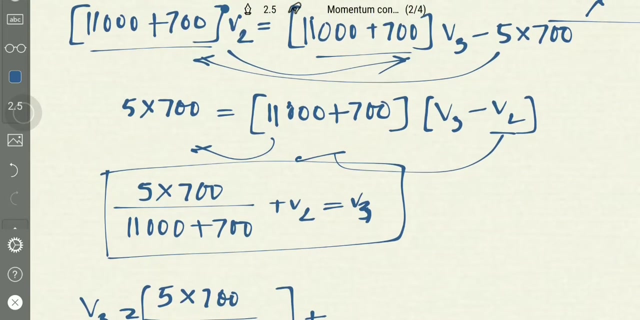 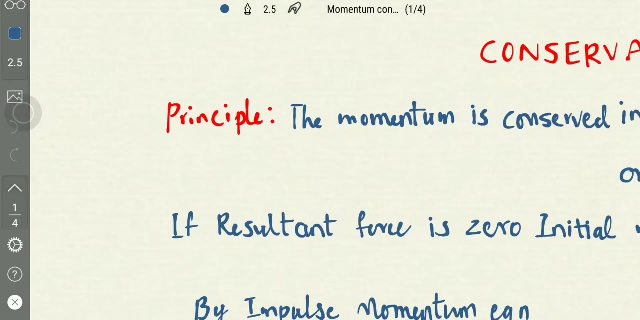 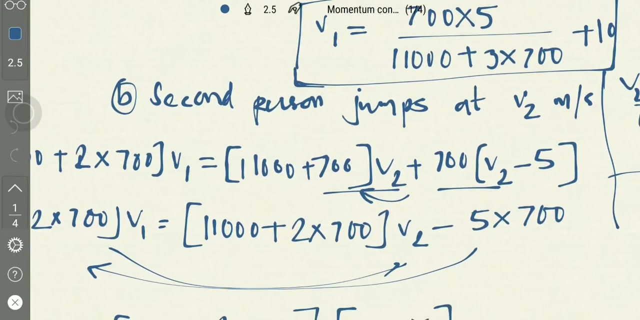 This is what V3.. So we know That, Finally, V3 is equal to 5 into 700. Plus 11000.. Plus What is V2.. We got V2 as 700 into 5 divided by 11000.. 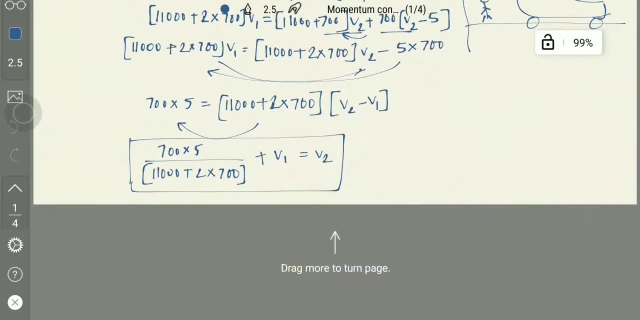 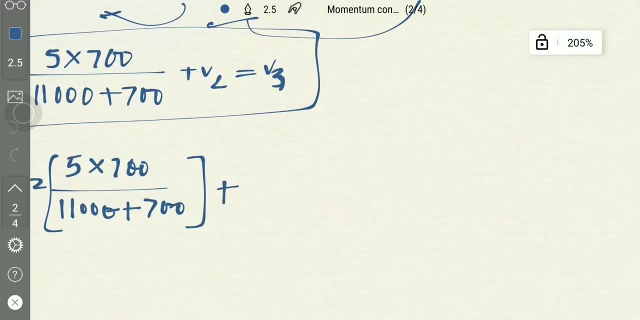 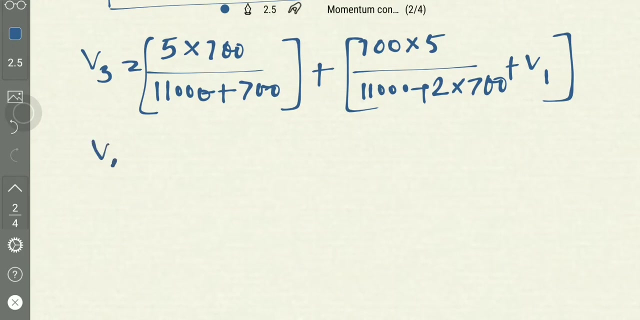 Plus 2 into 700, plus V1.. By substituting this Here, So V2, we got as 700 into 5. Divided by 11000.. Plus 2 into 700. Plus V1. And what is V1.? 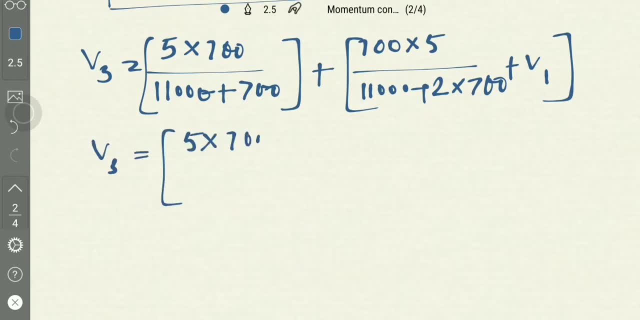 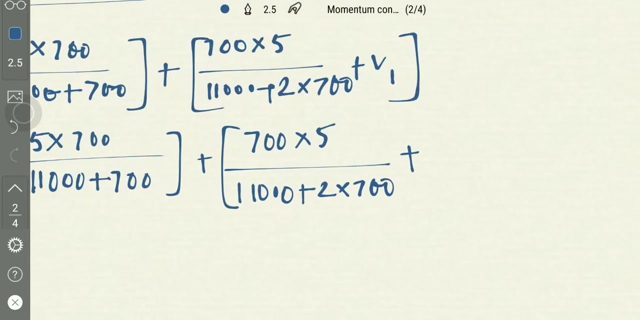 V3 is equal to 5 into 700, divided by 11000.. Sorry, 11000.. Plus 700.. Plus 700 into 5. Divided by 11000.. Plus 2 into 700. Plus. 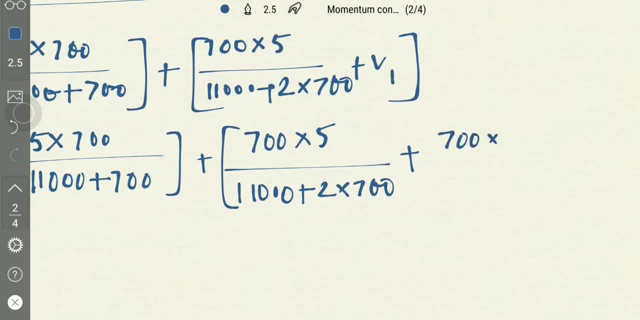 V1. we got it as 700 into 5. Divided by 11000.. Plus 3 into 700. Plus 10.. This is what V1.. This is V1. And if we solve this, We get. 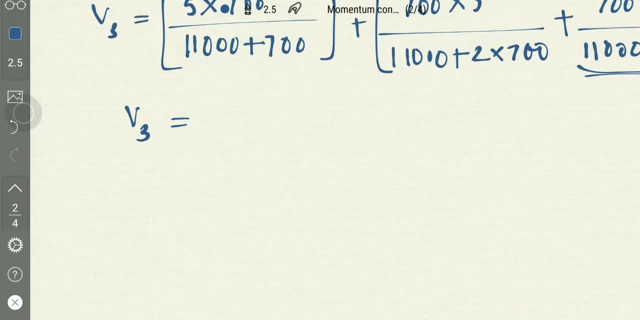 V3. As 10.849 meter per second. So this is what After After jumping one by one, The car travels with 10.849 meter per second. This is how we need to solve the Problems: using conservation of momentum principle. 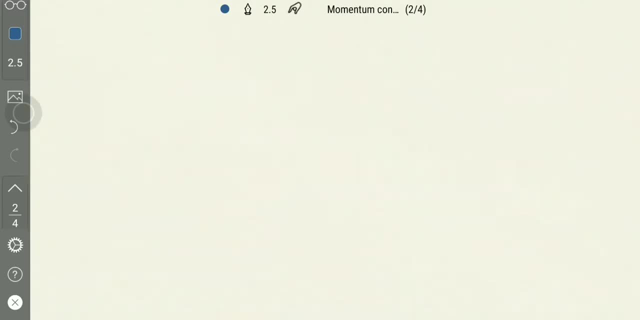 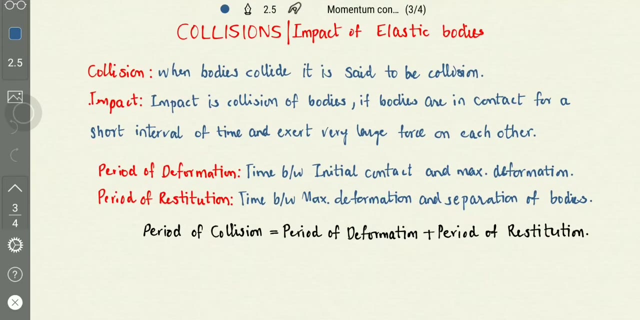 And now let us see Collision and impact of elastic bodies. Basically, what is collision? When Collide, It is said to be collision. Right When the bodies strike each other, That action is called collision. Then what is impact? Impact is a collision. 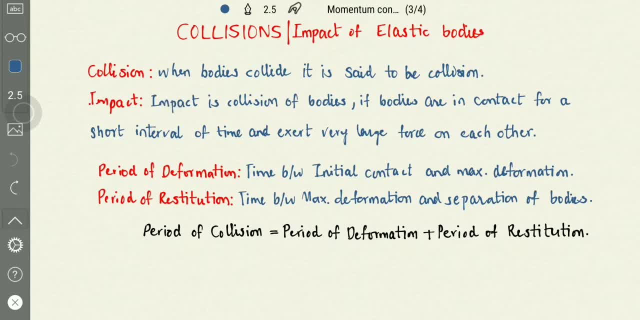 But. But during the collision The bodies are in contact for a short interval of time And exert very large force On each other. Then it will be called as impact, So The collision in which the Contact time is very less. 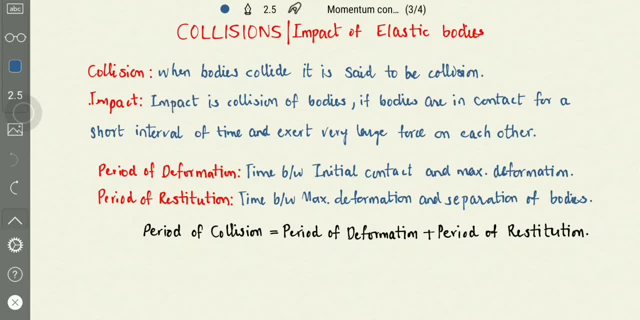 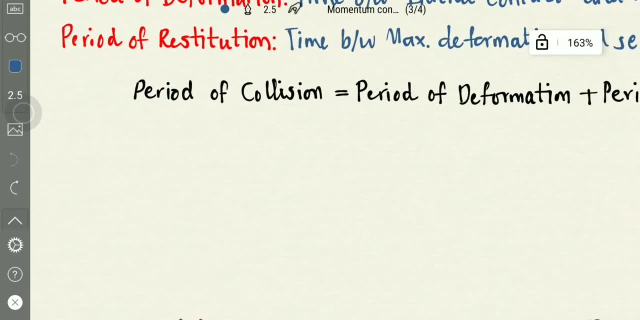 And the force exerted is very large Is called impact During collision. This happens like this: Modern elastic bodies Which deform. Elastic bodies are those Which deform And again It retains To Its original shape, Regains its original shape. 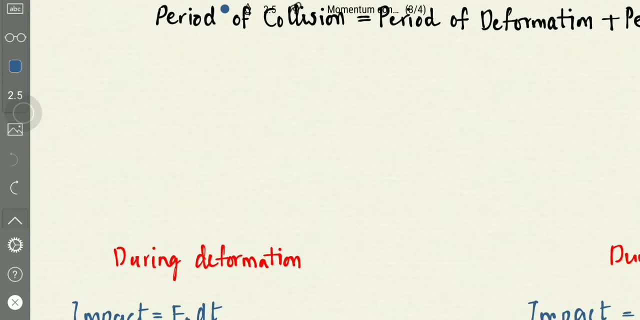 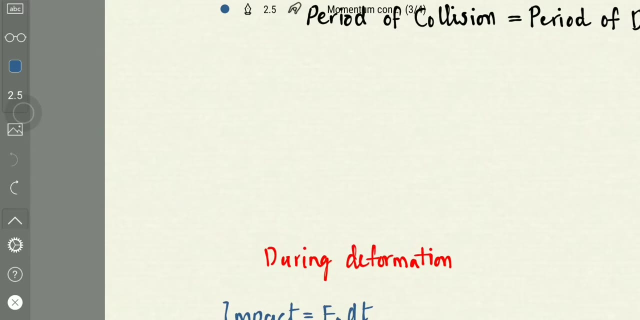 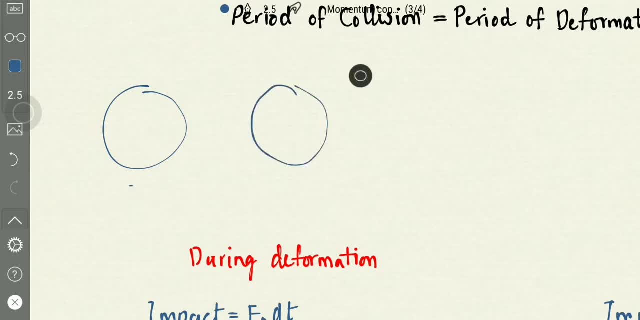 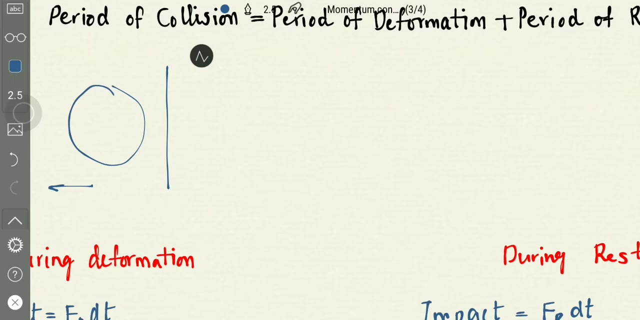 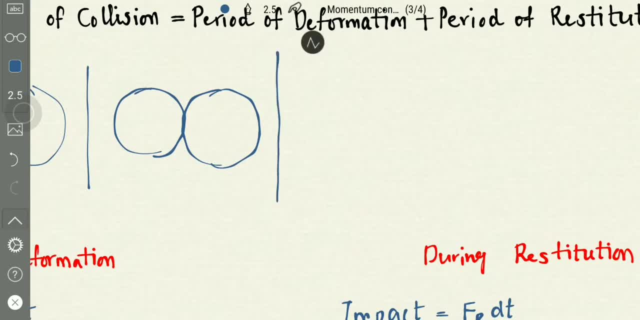 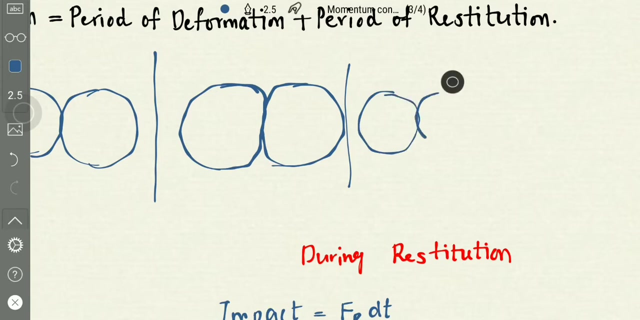 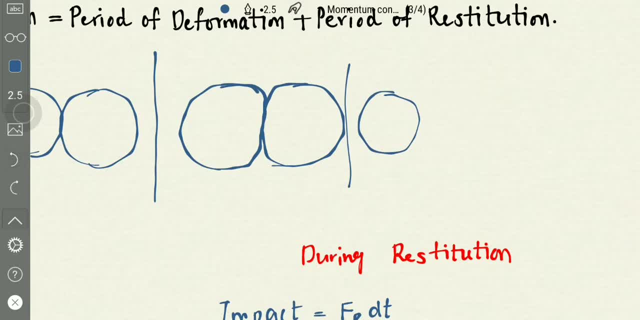 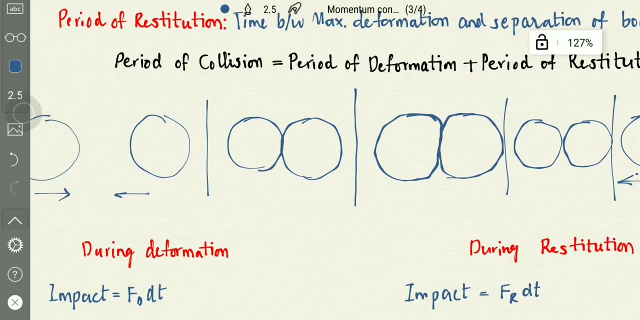 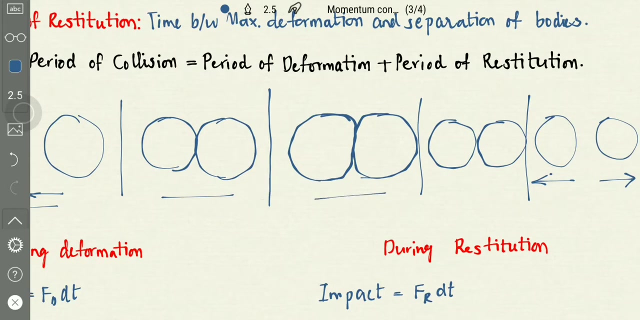 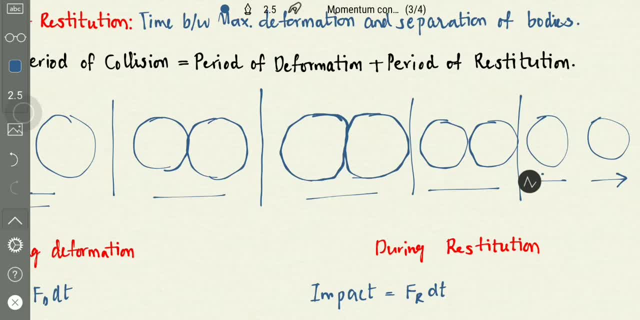 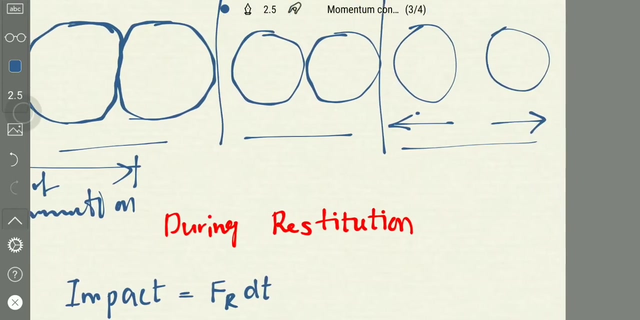 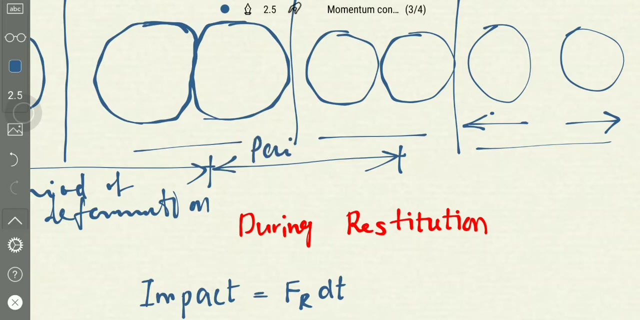 How, How, How? the contact, when they are going to separate, and this is separationThis period is called the period between the balls contacting and the maximum deformation is called period of deformation, and this is called period of restitution. period of restitutionThe period between initial contact and maximum deformation is period. 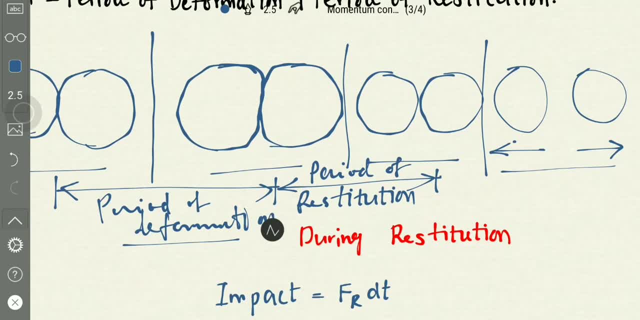 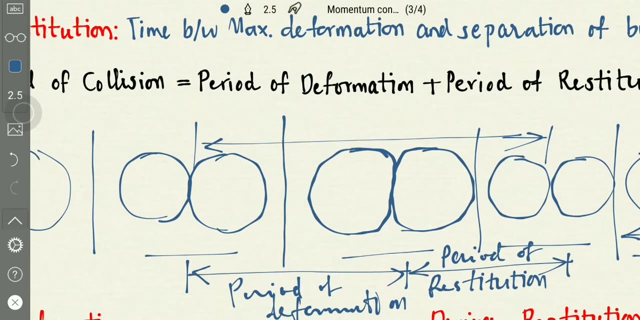 of deformation and maximum deformation, and period of deformation is period of deformation. Final contact is period of restitution. This total period is called initial contact to final contact is called period of collision. This is period of collision. So period of collision is sum of period of deformation and period of restitution. 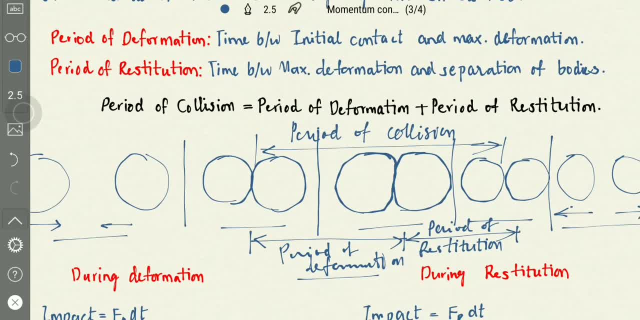 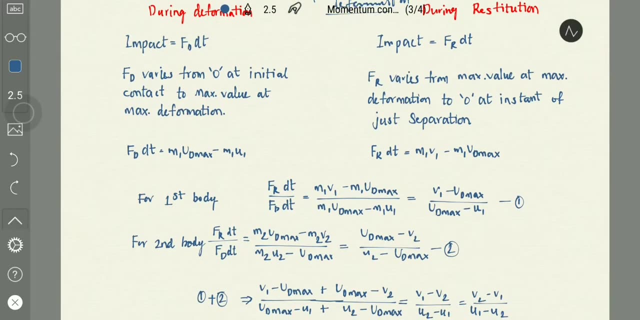 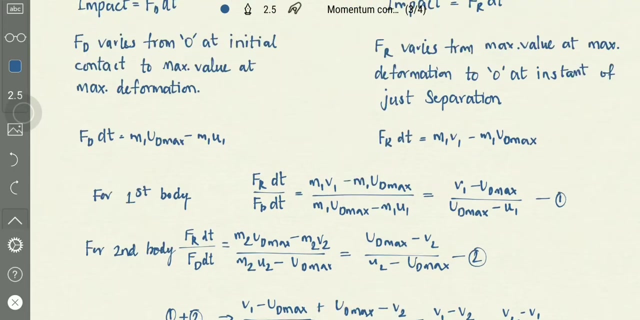 So what is period of deformation? Period of restitution is time between the initial contact and maximum deformation, and period of restitution is time between the maximum deformation and separation of the poles. So let us derive the equation which is called coefficient of restitution. In order to derive it, let us divide it into intersection surfaces. 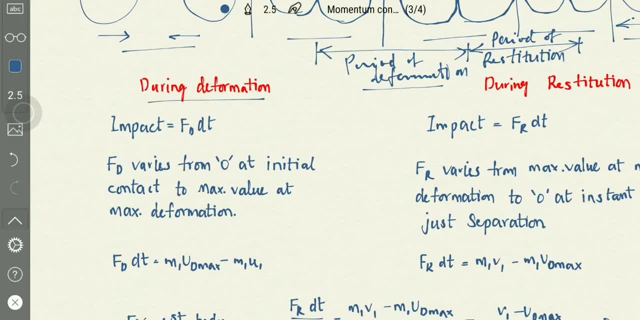 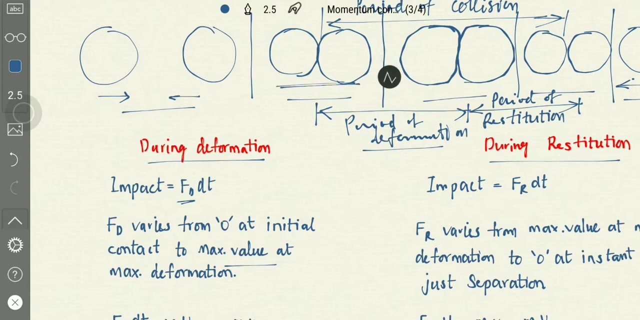 Let us divide the dre versus theSpeed, this into two parts: during deformation and during restitution. During deformation, let us say the impact is Fd. This Fd varies from zero at initial contact to maximum value at maximum deformation. So, as this is the initial contact, the force will be zero and when it reaches to a maximum, 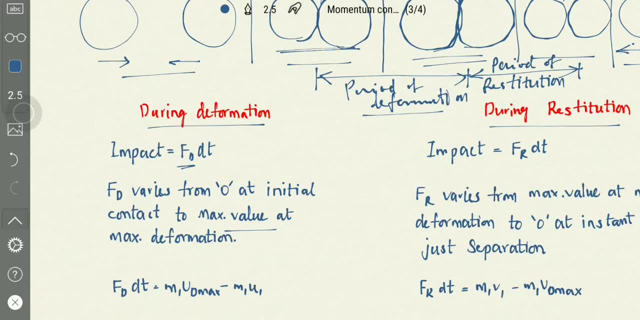 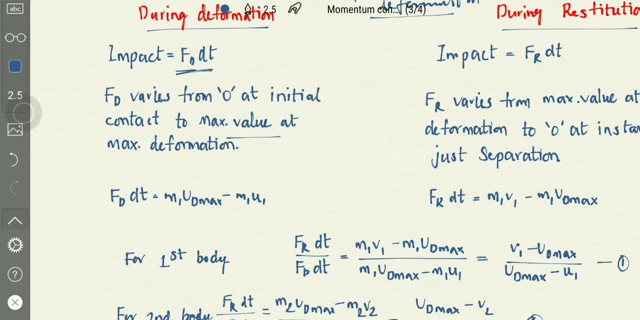 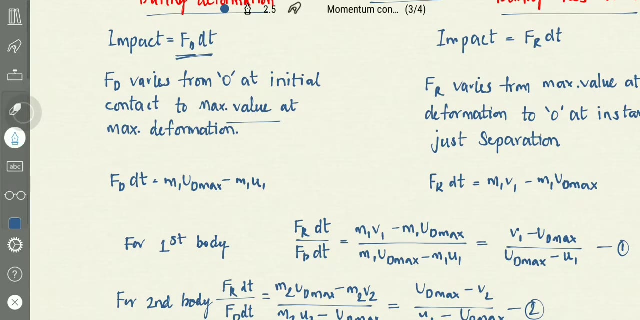 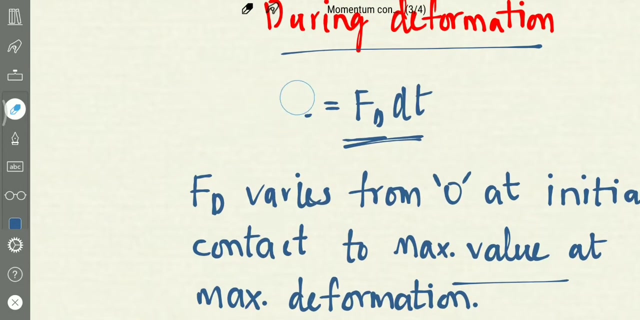 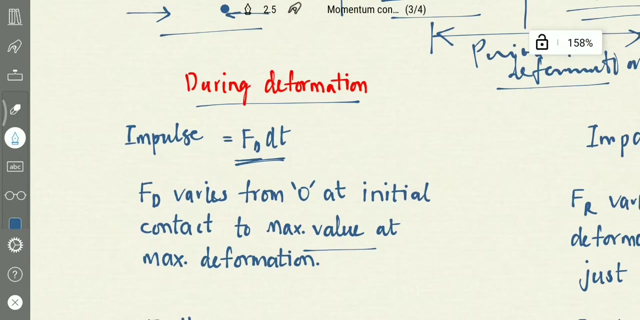 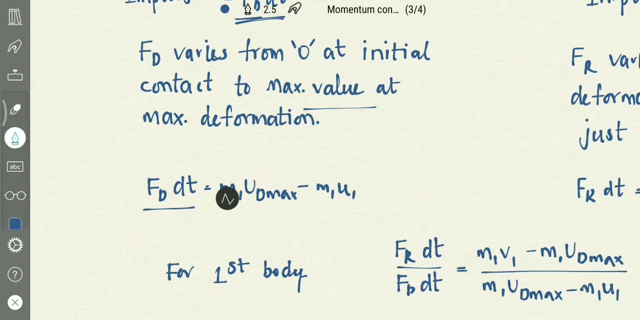 deformation, the force will be maximum. So the impact is Fd into dt. Sorry, this is impulse, This is impulse By impulse. momentum equation we get Fd into dt is equal to change of momentum: M1 Ud max minus M1 U1.. This Ud max will be same for first body and second body because the deformation 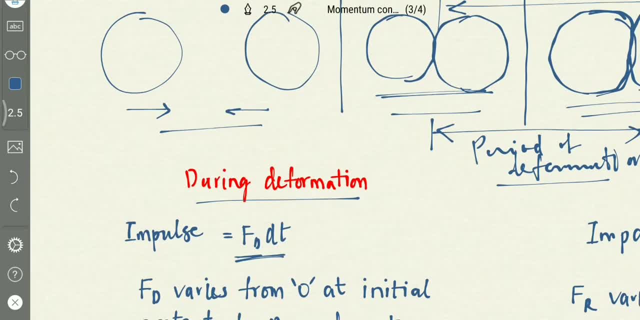 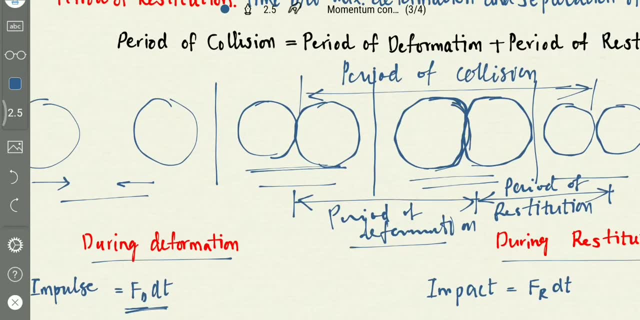 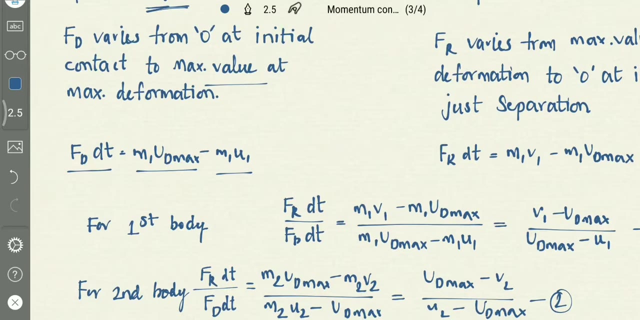 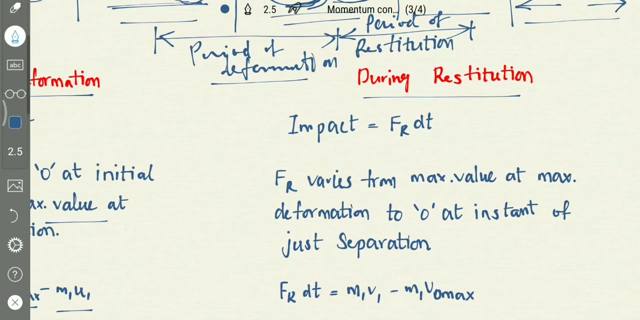 on the first body is equal to deformation on second body. So the velocity with which the velocity of when the deformation is occurring is constant, which is Ud max, And if you consider the restitution here also, it is impulse. Impulse is force into. 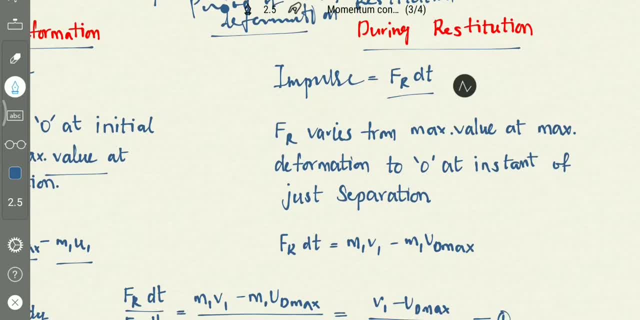 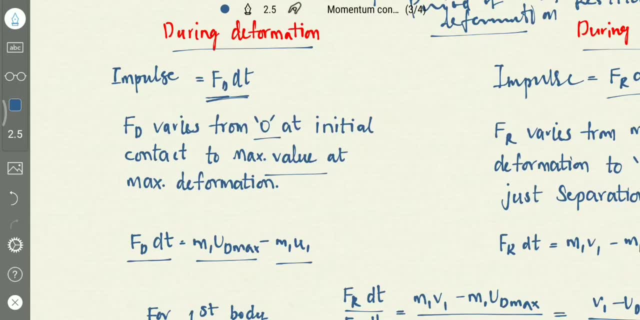 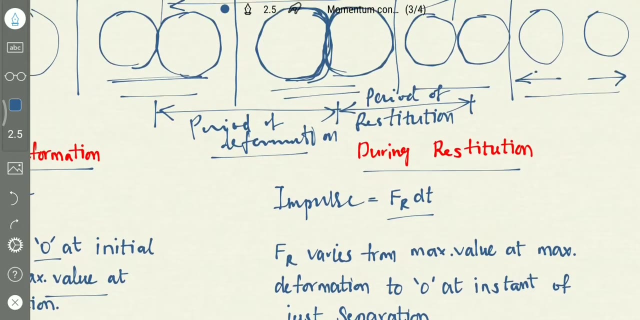 time right Fr into dt. Here we are not taking the total time because the force is varying In deformation. the force is varying from zero to maximum value at maximum deformation. and here, as it is restitution, this is the period of restitution. right, This is the period of restitution. Here the force will. 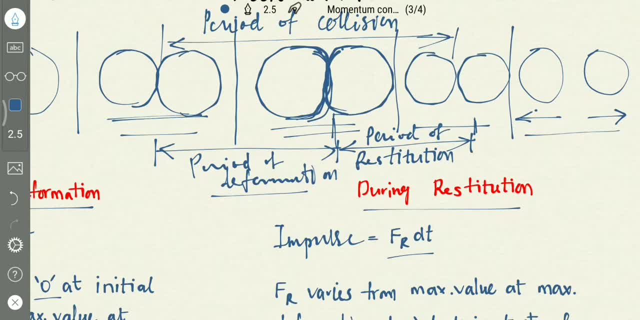 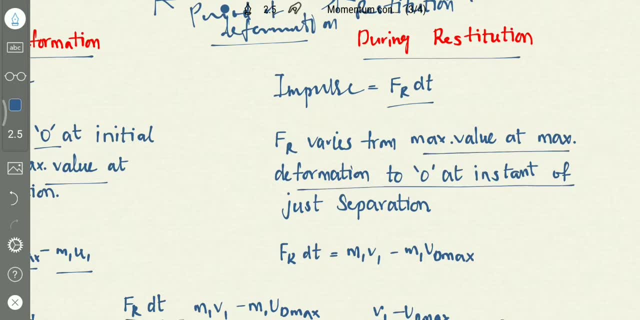 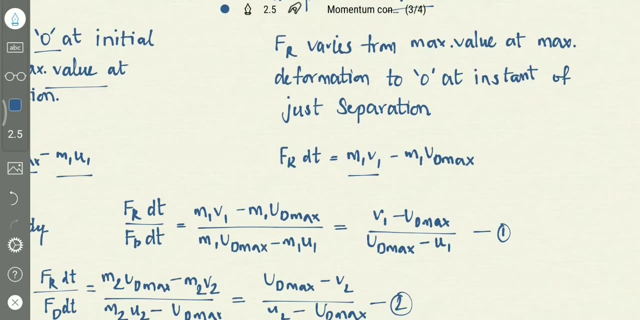 be maximum right. The force will be from maximum to a point minimum. The force varies from maximum value at maximum deformation to zero at maximum deformation. This is a to zero it instead of just separation. So fr into dt is m1, v1, sorry, final minus initial. 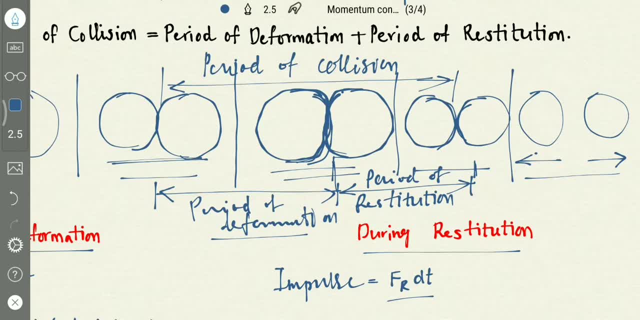 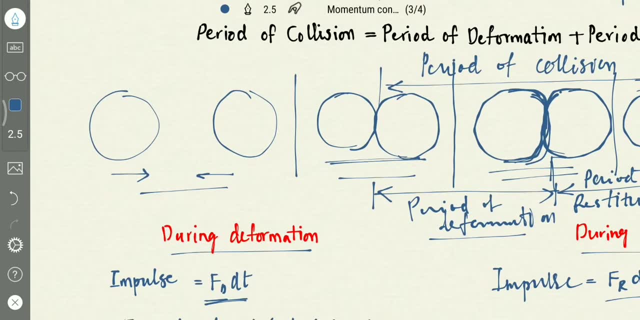 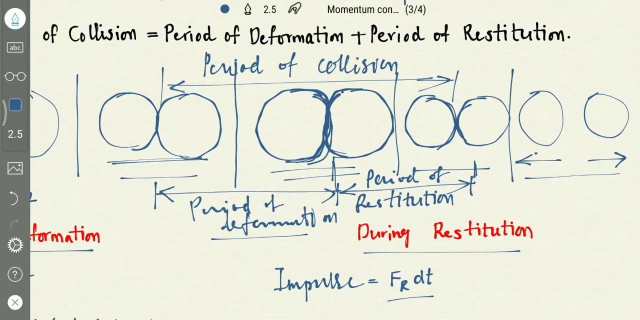 The final velocity, the final momentum is m1, v1, the velocity with which they are separating. So this is, let us say, u1,, this is u2, and here the velocity is, here it is udmax. udmax is the velocity and here it will be v1, here it is v2.. Final velocity of the body 1 and. 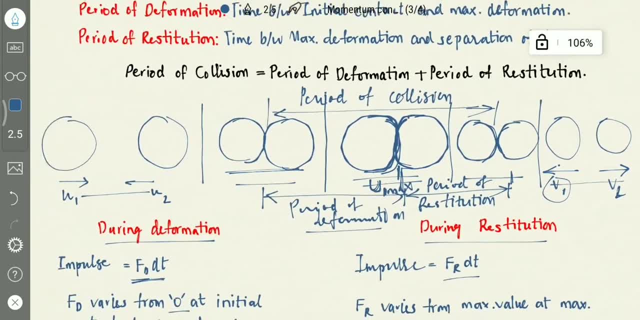 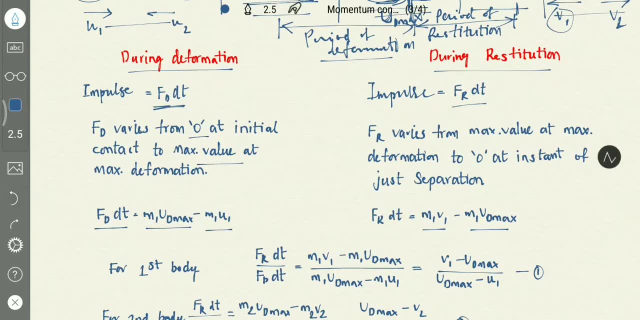 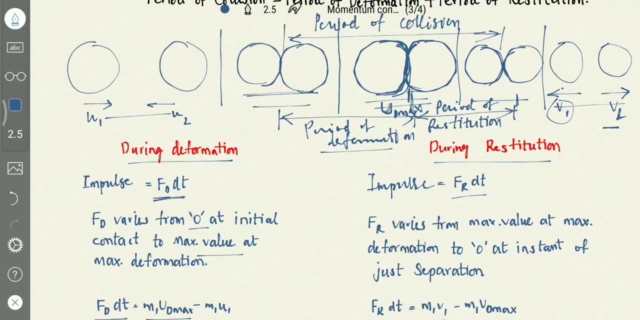 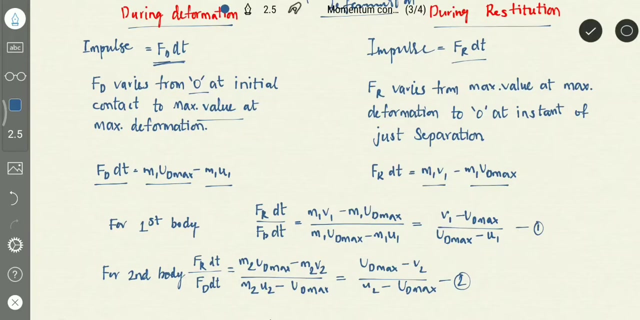 final velocity of the body: 2.. So it will be m1 v1, the final momentum is the final momentum. is this sorry? this is for the first body. just, we are considering only first body, m1 v1 minus m1 udmax, The. 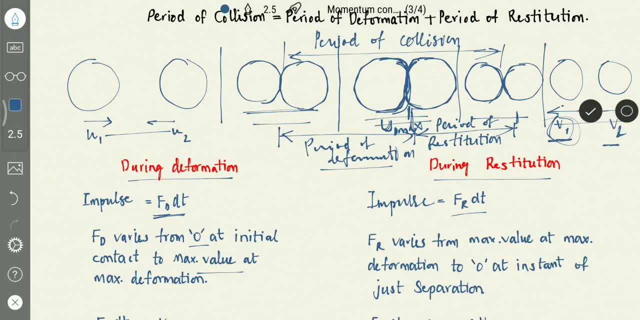 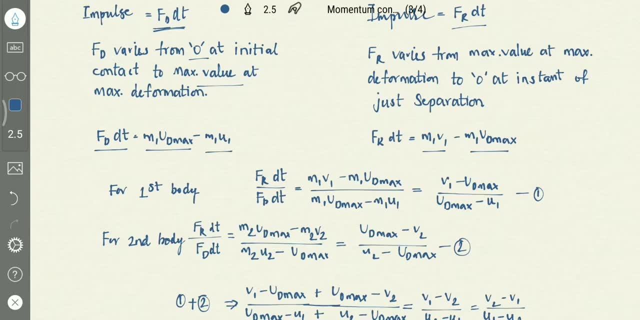 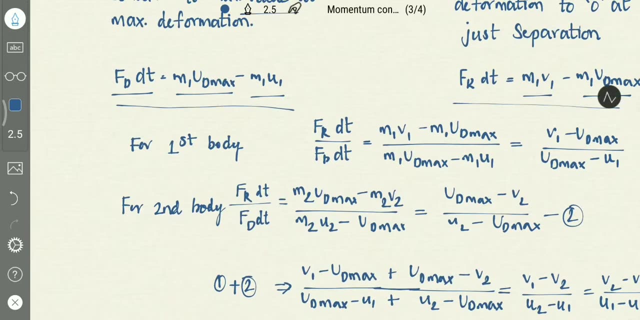 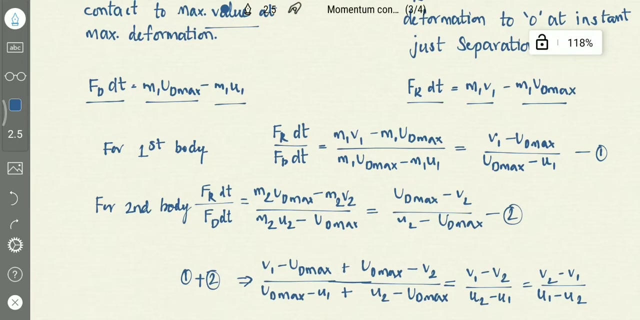 initial momentum for this period of restitution is this: m1 into u1.. Sorry, udmax. These are the equations for the first body And for the first body. if we divide, if we divide impulse for restitution and impulse for deformation, we get fr dt. 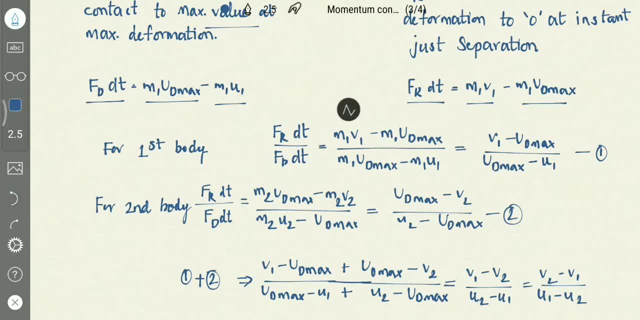 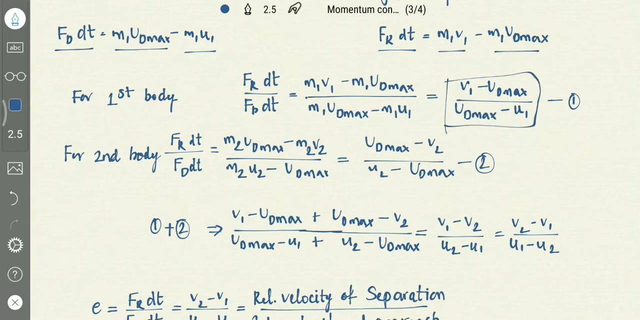 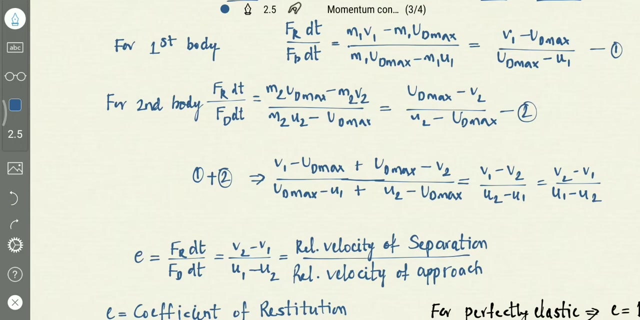 divided by fd dt, We get m1 v1 minus m1 udmax, m1- v1 minus m1 udmax. And if we take common m1, m1 gets cancelled and we remain with v1 minus udmax divided by udmax minus u1.. Similarly, if we consider for second body, it will be m2 udmax minus. 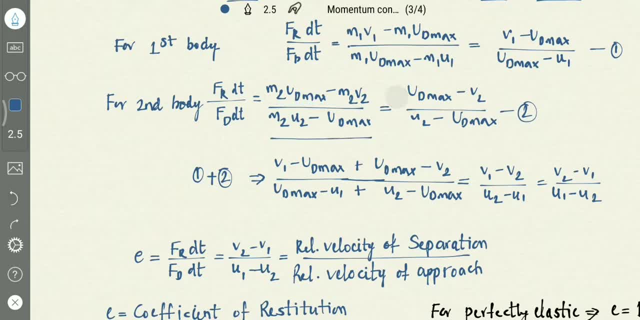 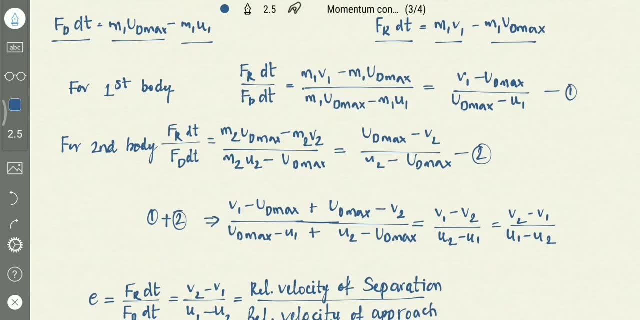 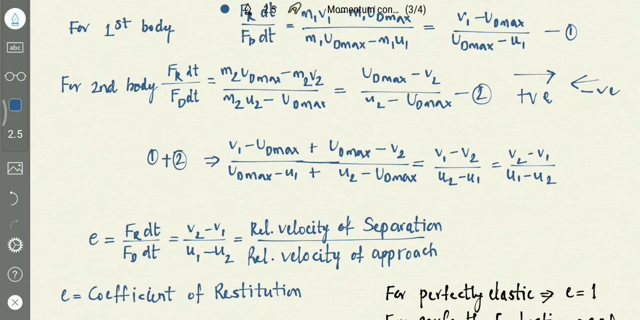 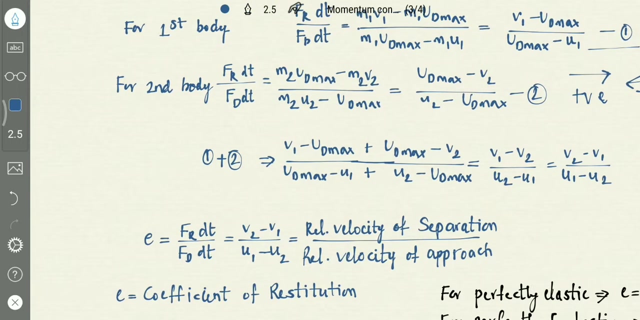 m2 v2 and m2 u2 minus udmax. We get this by considering the rightward direction as positive and left as negative. So this is equation 1 and this is equation 2.. In order to get for both the bodies, this is for the first body and this is for the 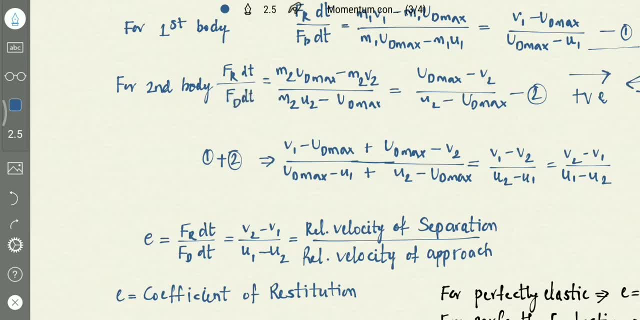 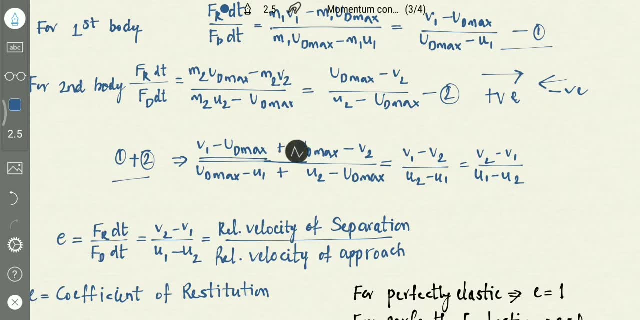 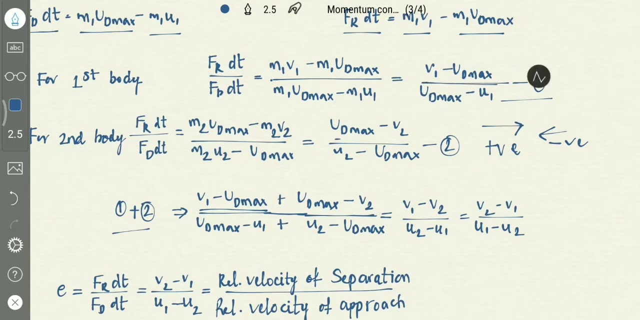 second body. So total impulse ratio is given by 1 plus 2.. This will be V1 minus Udmax, plus Udmax minus V2.. Here you can see V1 minus Udmax, Udmax minus V2.. This is what we wrote here and in the denominator: Udmax minus U1 plus U2 minus Udmax. 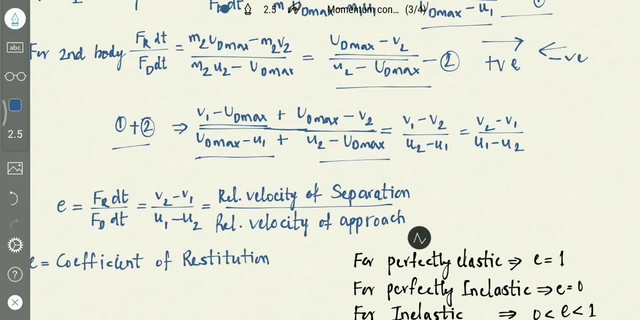 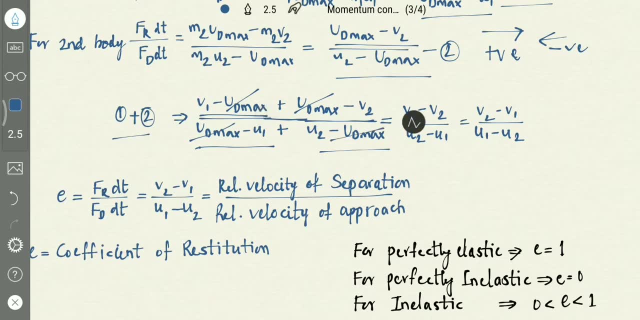 Udmax minus U1 plus U2 minus Udmax, We get this Udmax, This Udmax minus U1 plus U2 minus Udmax. Udmax gets cancelled. here and here again it gets cancelled. So we remain with V1 minus V2, divided by U2 minus U1, and also we can write it as V2 minus. 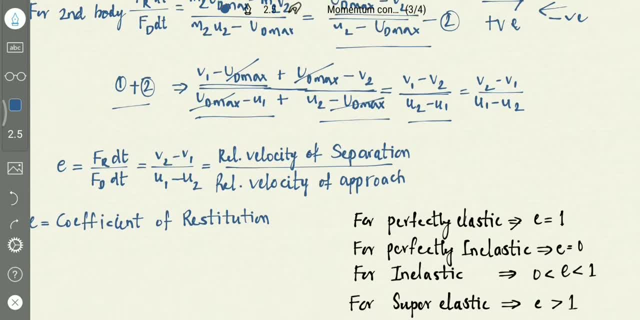 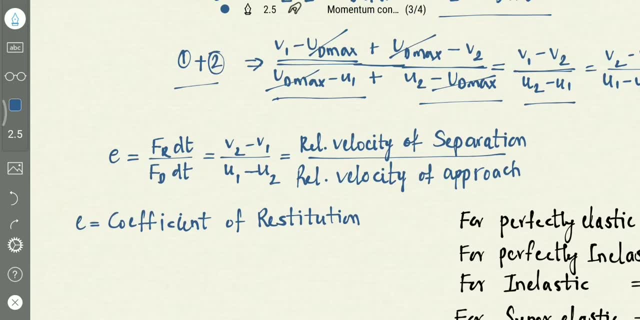 V1 by U1 minus U2 by changing the signs on numerator and denominator, And this is called coefficient of restitution. This is the ratio of V2 minus V1 and U1 minus U2 is called coefficient of restitution, This V2 minus V1, what is V2 minus V1?? 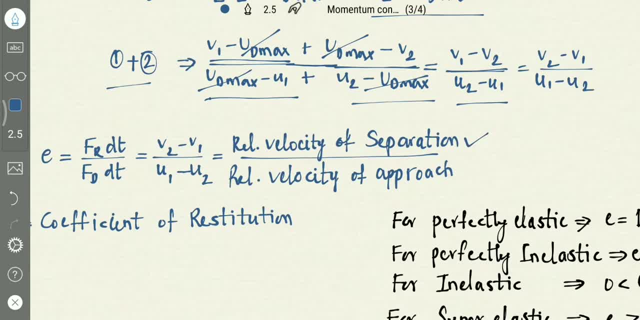 The final velocity minus initial velocity, which is relative velocity of sorry. This is velocity of the final velocity of the second body minus initial sorry. final velocity of the first body, which is velocity, relative velocity of separation. And if you consider two bodies before impact, 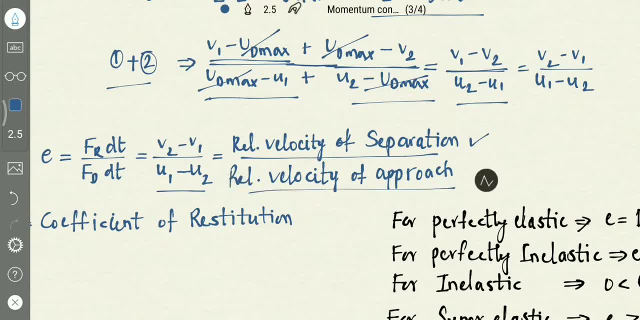 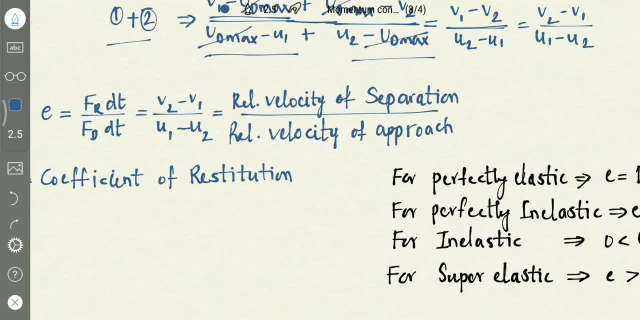 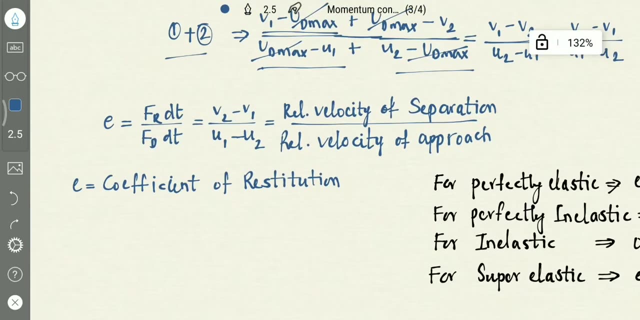 Velocity is of two bodies. before impact It will be relative velocity of approach. So V2 minus V1 is relative velocity of separation which is after the impact, And U1 minus U2 is relative velocity of approach which is before the impact. And this E is called as coefficient of restitution. 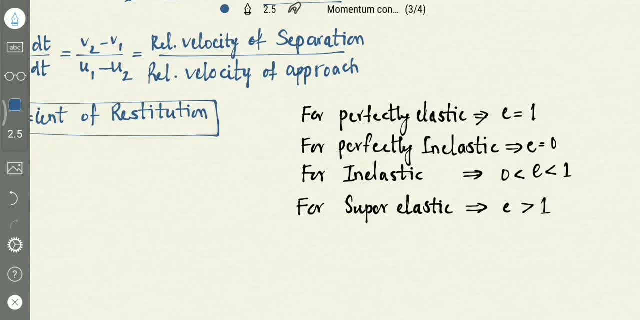 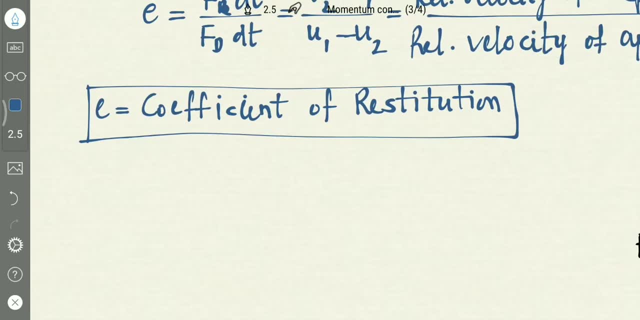 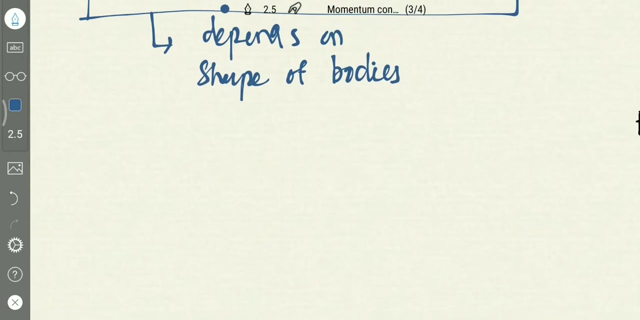 And this E depends on shape of E depends. this E depends on Depends on shape of the bodies, shape of bodies, And again, material, material of bodies, etcetera. It may depend on many factors, But these are the important. 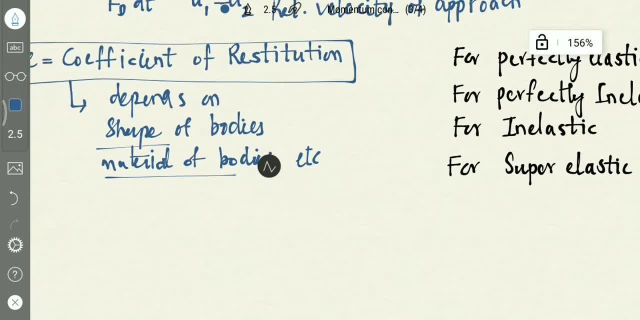 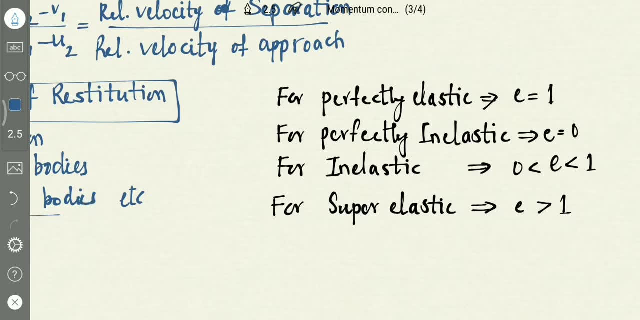 Shape of the bodies, Etc. Shape of the bodies and material of the bodies. And for this is the important one, It may be asked for one mark. So for perfectly elastic, perfectly elastic bodies, E is equal to 1 and perfectly inelastic. 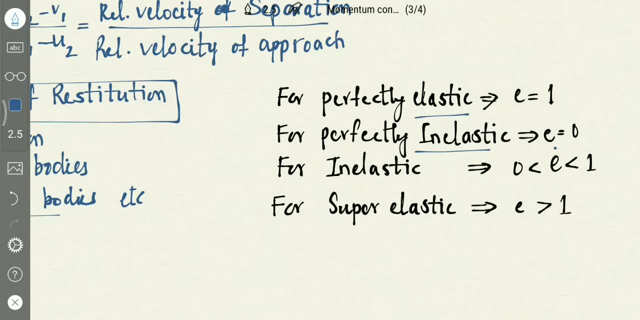 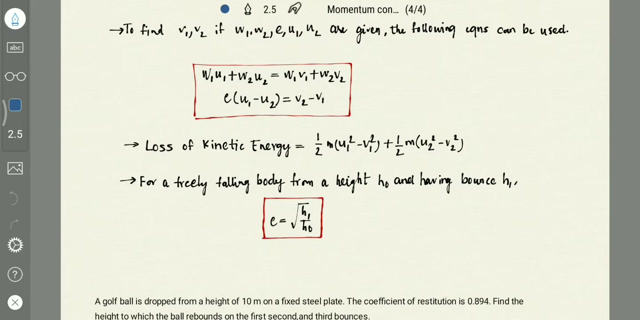 or it can be said as perfectly plastic bodies, E is equal to 0 and, perfectly sorry, for normal inelastic bodies it will be 0 to 1, and not including 0 and 1 here, And then Super elastic bodies, E will be greater than 1.. 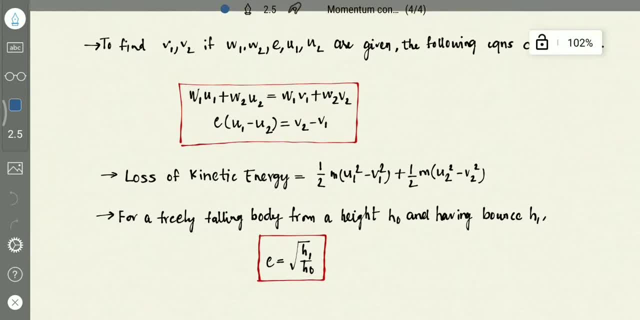 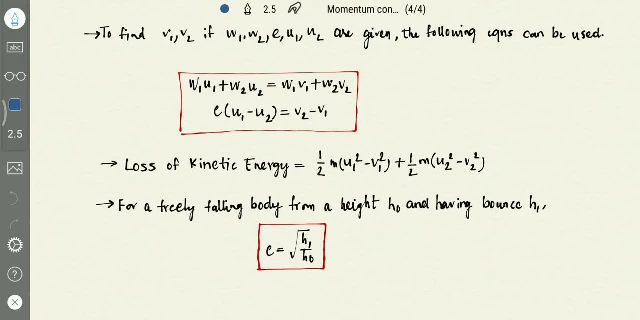 So, for this, summing up the collision, there are three important formulas which we can. by this, we can apply directly to the wave, For example, W1, W2, E, U, U1 and U2.. What are these? 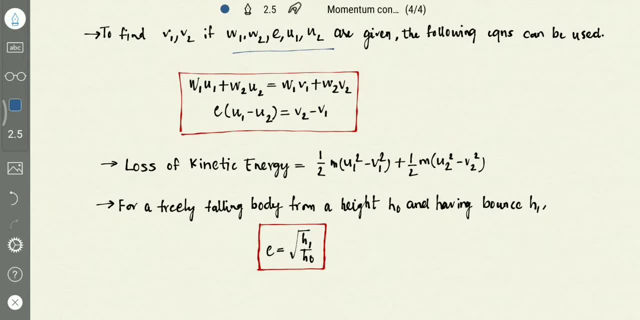 W1, W2 are weights of the bodies, E is coefficient of restitution and U1 and U2 are initial velocities of first body and second body. If these are given and it is asked to find V1 and V2,, then the following equations can: 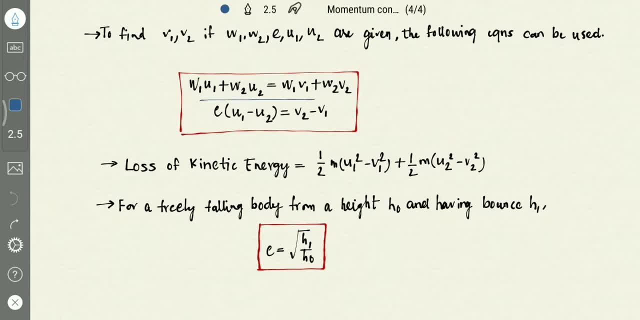 be used. What are those equations? This: W1, U1 plus W2, U2.. Which is equal to W1, V1 plus W2, V2.. This is what is this Conservation of momentum. And E into U1 minus U2 is equal to V2 minus V1. 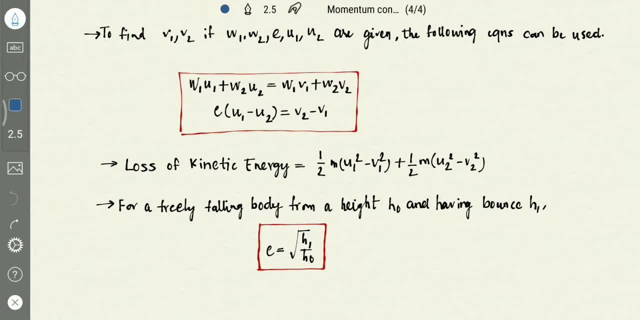 We have seen coefficient of restitution formula as V2 minus V1 by U1 minus U2.. Taking U1 minus U2 to LHS from RHS we get this. So these two equations can be used. This is conservation of momentum equation. 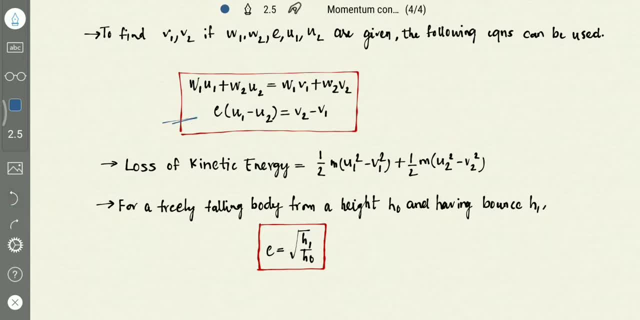 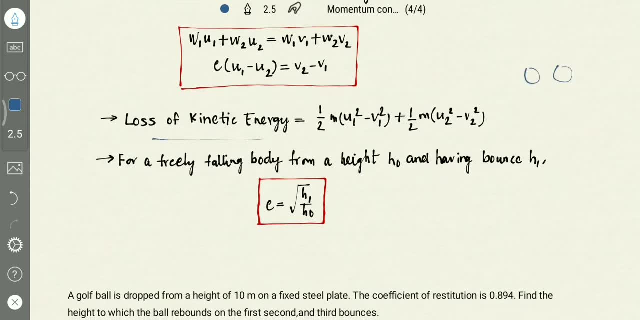 And this is conservation of momentum equation. This is, we got formula as coefficient of restitution And during the impact, during the impact there will be a loss of kinetic energy. So what is the loss of kinetic energy? Kinetic energy is given by half mv square, half into mass, into velocity square. 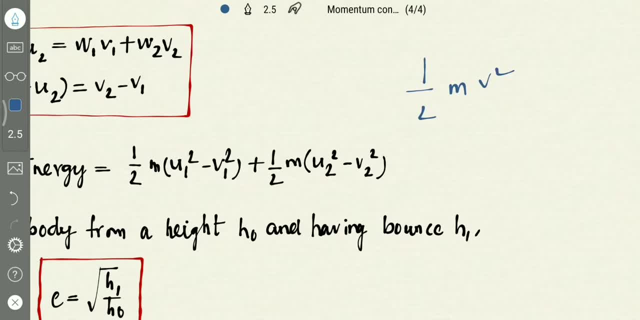 The kinetic energy loss will be by both the bodies. right, The first body losses a velocity of half m. Initially it will be high, minus half mv1 square. The final velocity will be less than initial velocity right. So it will be half mv1 square minus half 1v1 square. 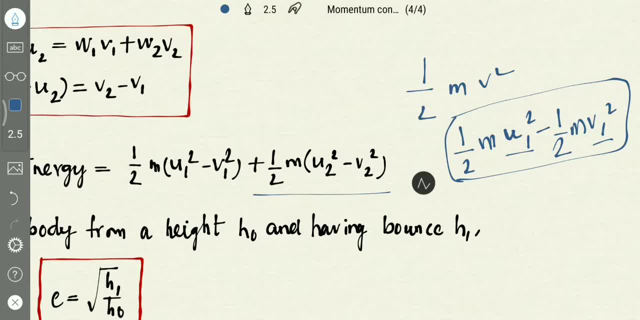 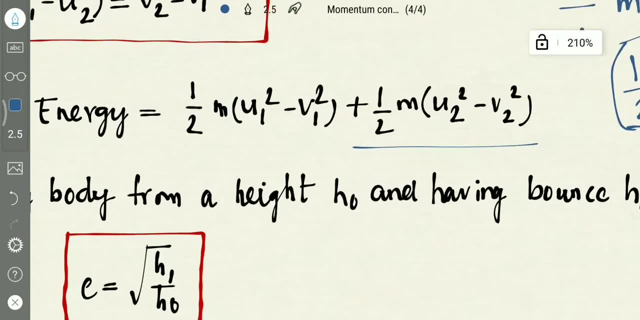 And similarly for second body, it will be half m U2 square minus V2 square. This also can be written as if the bodies are detained half, As wasn't there right? This will be my test. Thank you, That was my test. 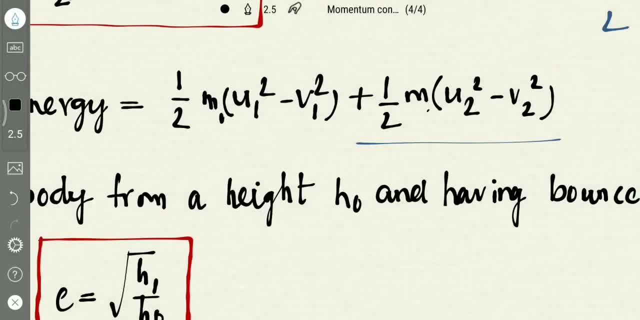 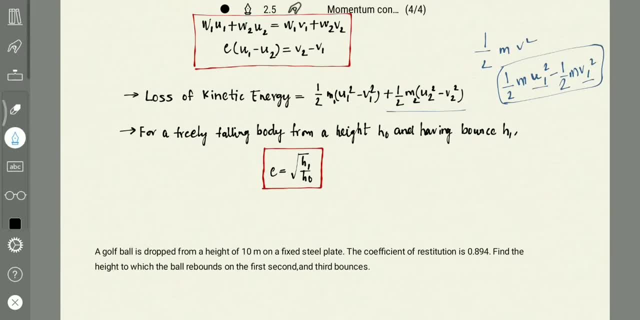 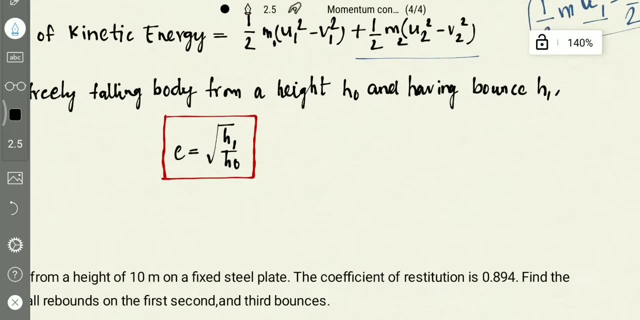 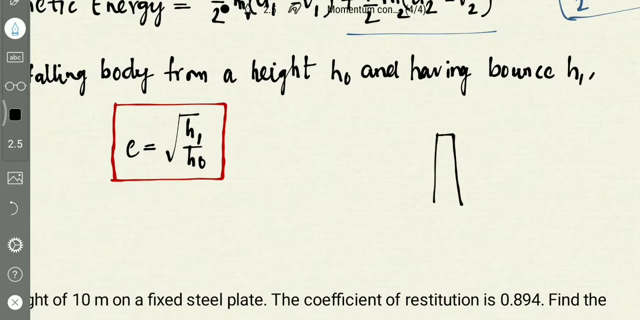 Okay, Bye, bye with different masses, it will be m1 and m2. and there is one important formula for a freely falling body: from a height h0 and bounce h1, e is equal to. so if there is a- let us say there is a tower from which a body is dropped, and this height is h0, and it rebounds us to 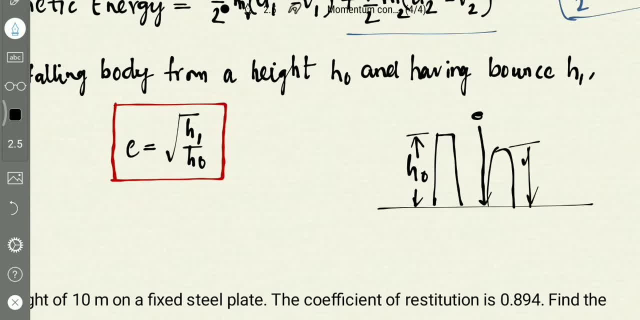 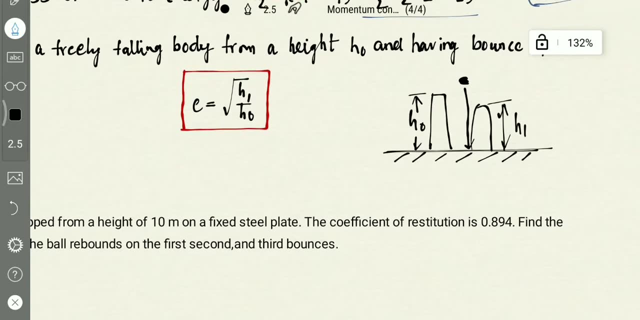 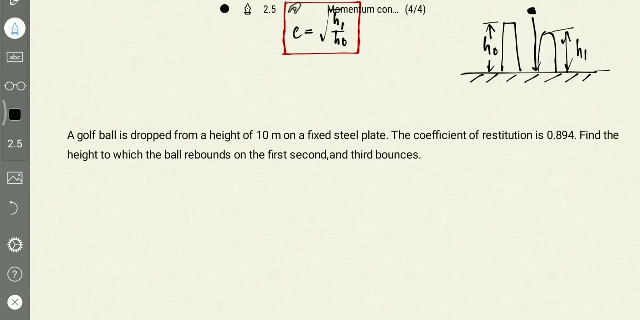 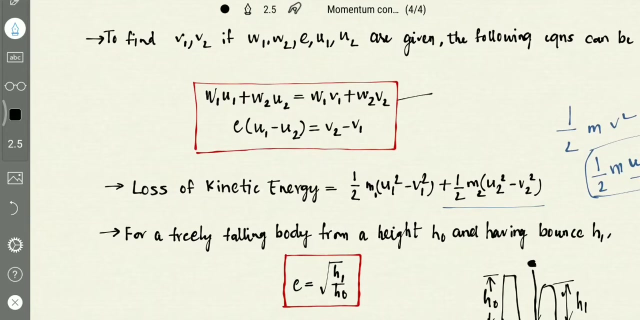 a height h1, then the coefficient of restitution between this body and this surface is equal to, under root, h1.. h1 by h0. the derivation is not required, as gate is based on answers and not the derivations. So these are three important formulas. first one is the conservation of momentum and the 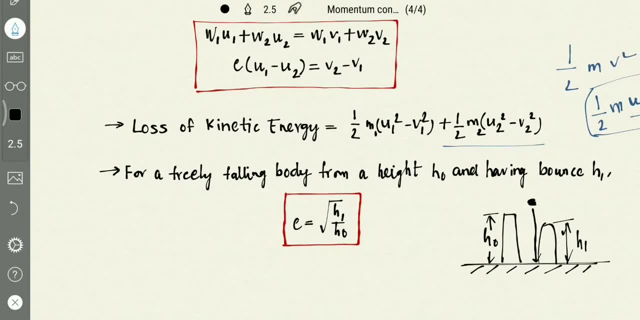 second one is coefficient of restitution based formula. and next one is loss of kinetic energy: how much kinetic energy is lost during the collision? and next one is for a freely falling body, h1, and having a bounce: what is the coefficient of restitution between the body and the surface? 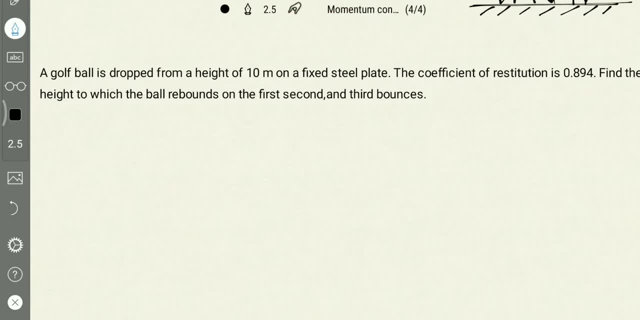 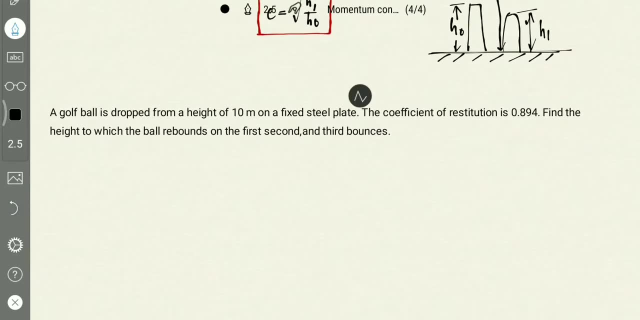 on which the body is hitting. Let us solve this problem based on this formula. See, there is a golf ball is dropped from a height of 10 meters on a fixed steel plate. the coefficient of restitution is 0.894. find the height to which the ball rebounds us on. 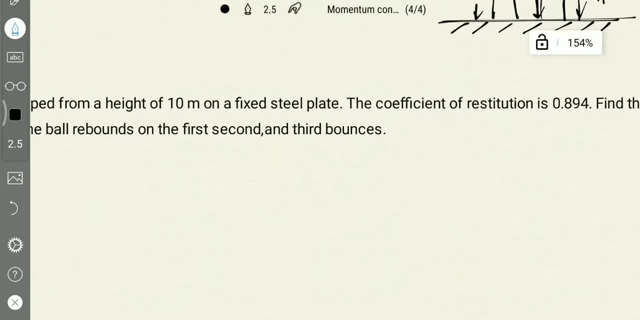 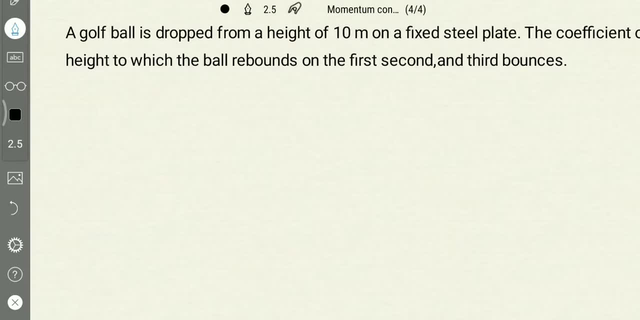 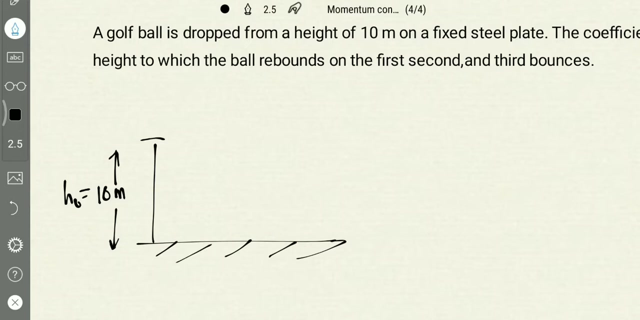 first, second and third bounces. So he is asking us to find, on three bounces, what is the height reached. First, it will be dropped from 10 meters height. this is 10 meters, and it is h0. this is the steel plate, fixed steel plate. and then it rises to a height of- let us say it is h1, and again. 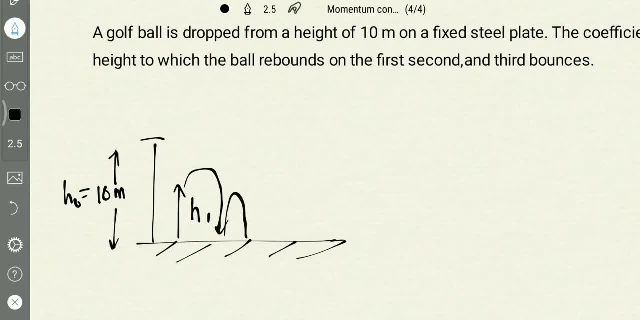 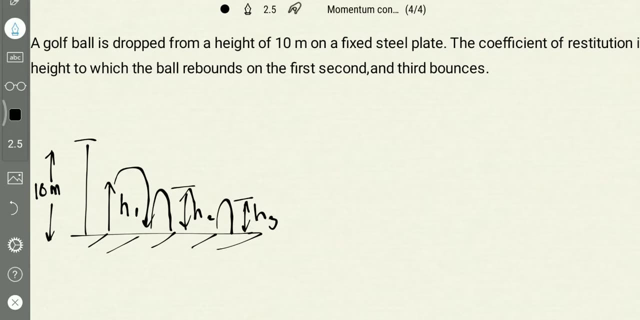 it falls. again it rises to a height h2. again it rises and falls, it is h3.. it is asked to find the three heights right: 1st, 2nd, 3rd bounce. 1st one, this is second bones and this is third bones. Firstly, we know E is equal to under root. what? 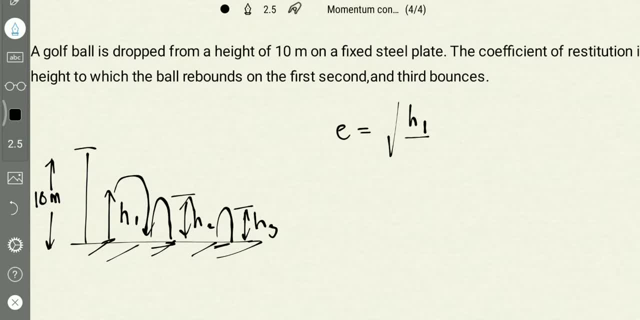 is the formula: h1 by h0, right, h1 by h0.. This is the formula and we need to get the answer. from this, h1 is equal to E square, squaring on both sides and multiplying h0 with E square, and from this we get h1, as h1 is equal to what is coefficient of restitution. 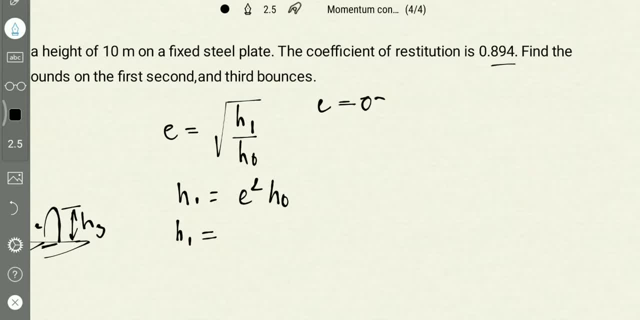 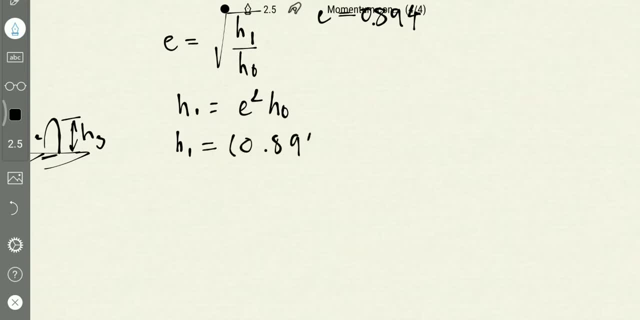 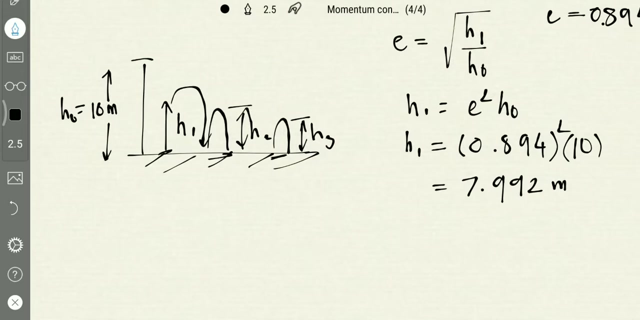 E is equal to 0.894.. So it is 0.894 square into what is the initial height. It is 10.. We get h1 as 7.992 meters, And what is next one? This will become h1.. So E is equal to under root and the next one. 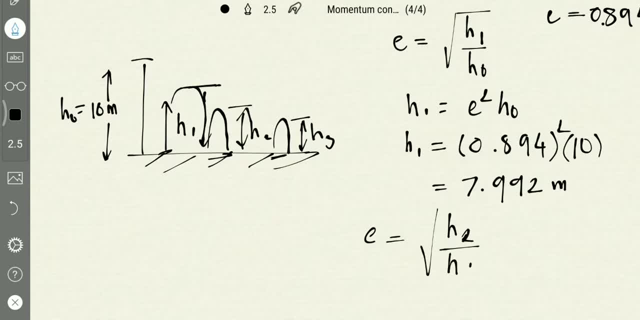 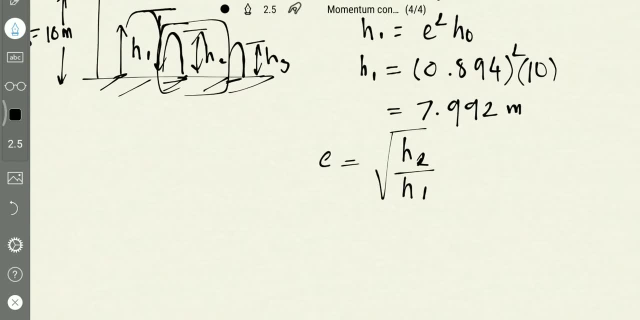 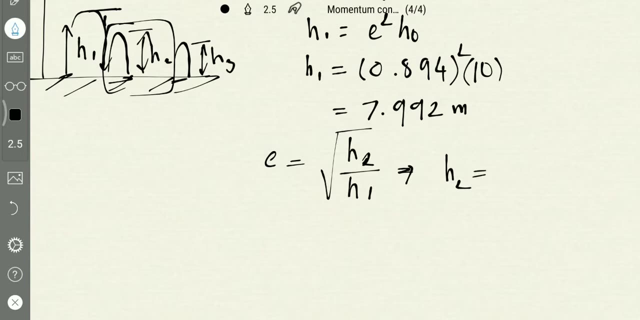 will be h2 right, h2 divided by h1.. And for this it will become h2 by h1.. We need h2 right. h2 is equal to E square into h1.. And h2 is equal to what is E 0.894 square. 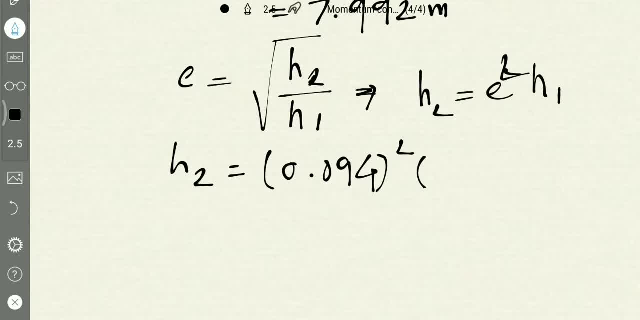 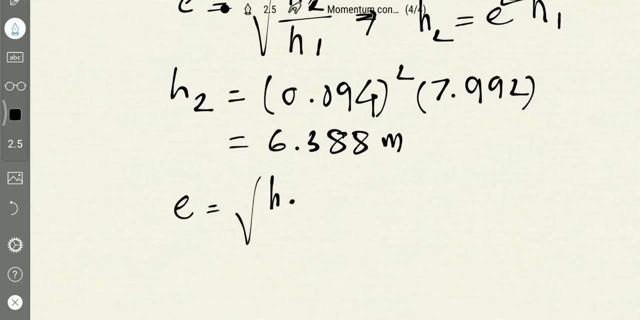 0.894 square into what is h1? 7.992.. We get h2 value as 6.388 meters And the next one is the E is equal to under root h3 by h2.. We get h3 as E square into h2.. So 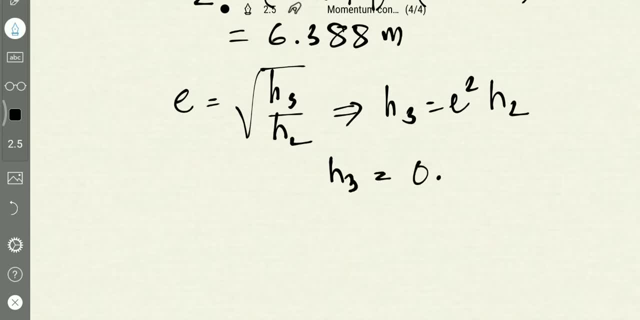 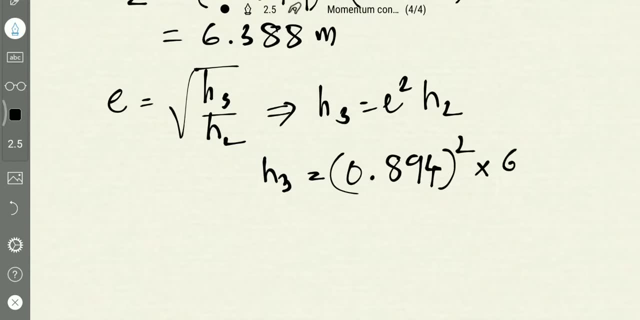 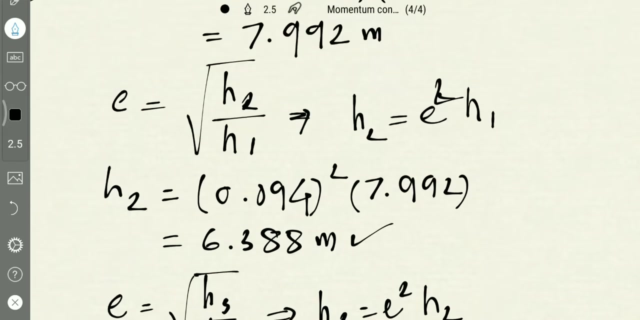 h3 is equal to 0.894, square into h2 is 6.388 and we get h3 as 5.105 meters. This is the third bones one. this is the second bones and the first one is 7.992 meters. 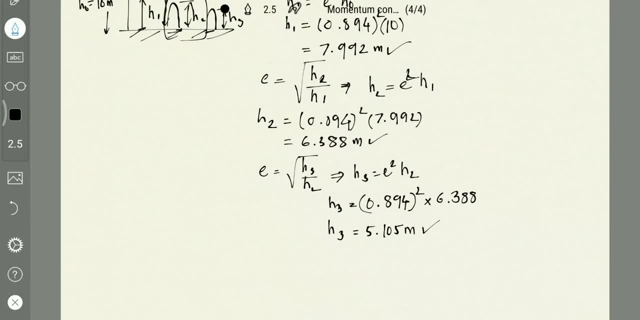 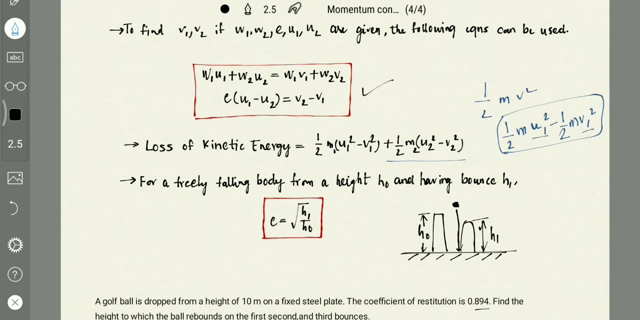 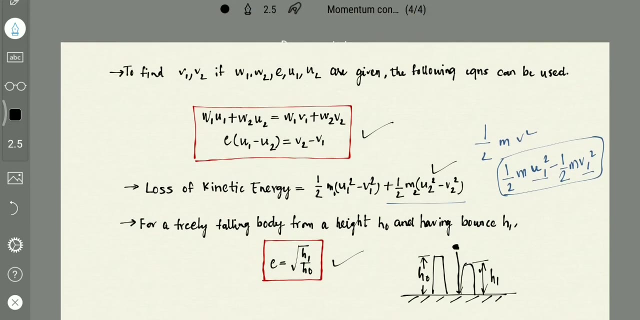 This is how we need to solve the problems. based on collision, The problems may be asked based on this one and based on loss of kinetic energy or this. So you need to practice the problems. I will attach the problems with this video in the description. 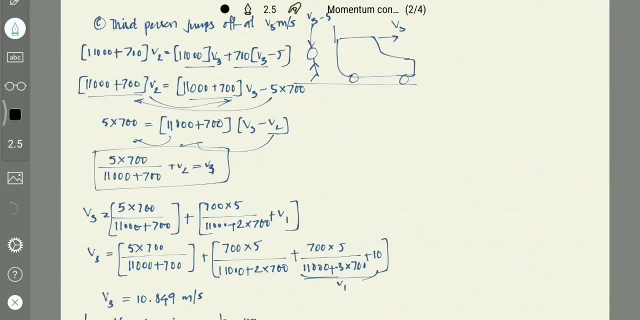 So you can practice more problems. So if you like this video, please like, share and subscribe this channel. Thank you.